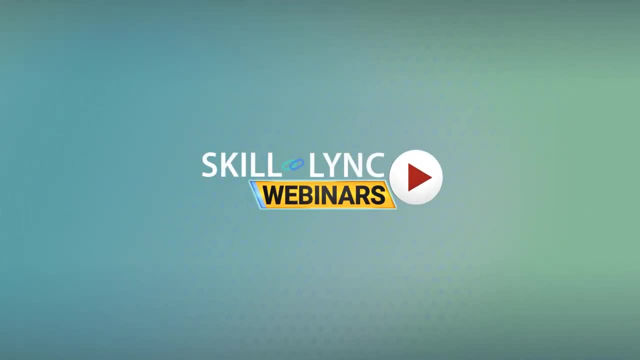 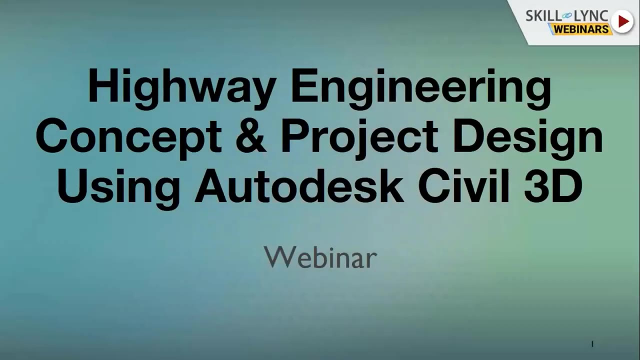 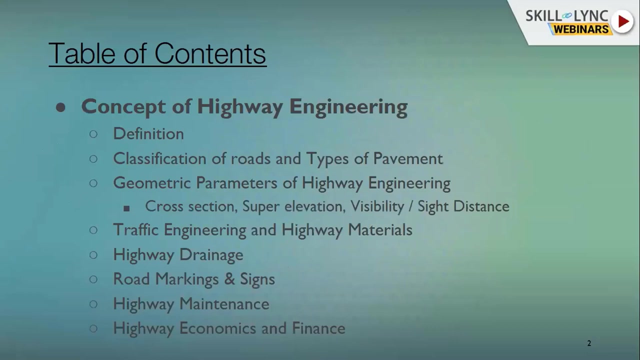 So, before starting, I would like to give you a brief about what we are covering in this presentation. So the first and foremost will be the concept of highway engineering. In this one, I am trying to explain you about the highway engineering concept, what it is. 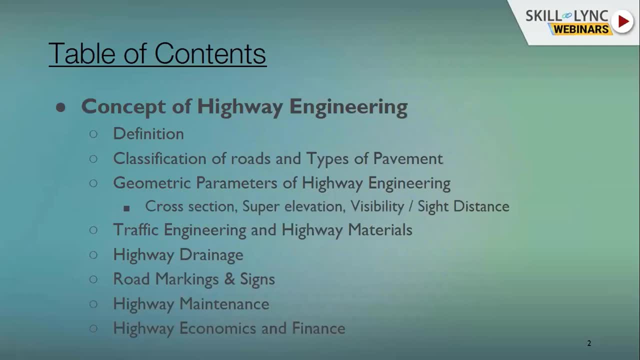 what are the different kinds of parameters we use in the technical terms for highway engineering? First it will be a definition of highway engineering. Next I will be explaining the classification of the roads and different types of pavements and the geometric parameters which we involve in this highway engineering to design a project which has the subparts. 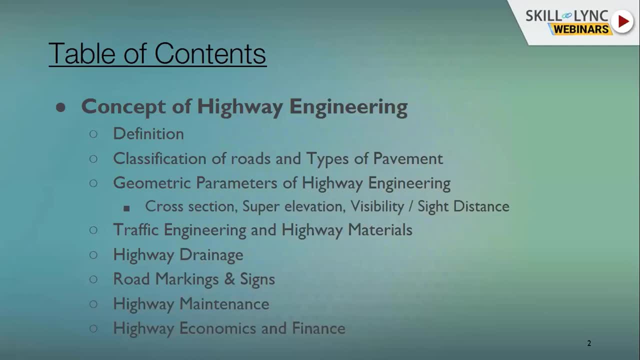 as well, like cross-section super elevation visibility outside distance. So those are the parameters. I was just briefing up And moving along. we just also see through the basics about traffic engineering: highway materials design, highway designs, highway drainage, road marking and signs- highway. 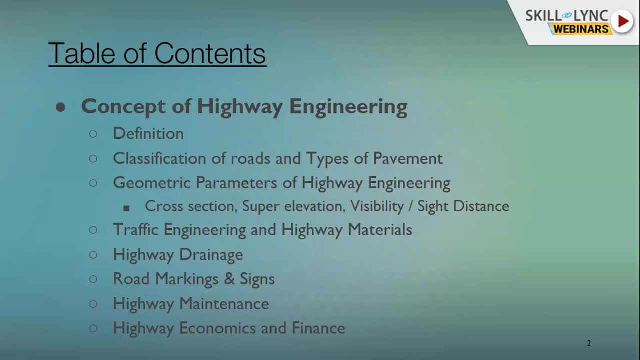 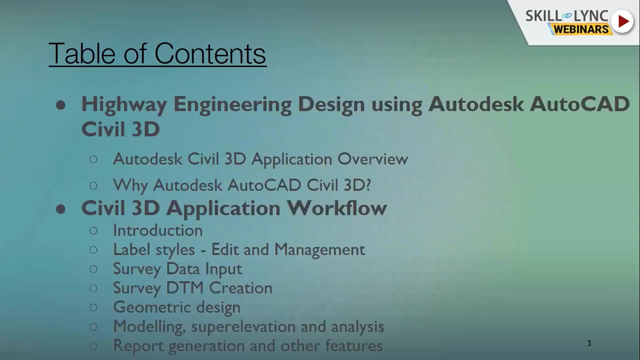 maintenance and how it helps in economics and finance in a region or for a country as a whole. So those are the parameters. about highway concept, I will be trying to explain you in this presentation. So, moving along after the brief introduction about highway engineering, 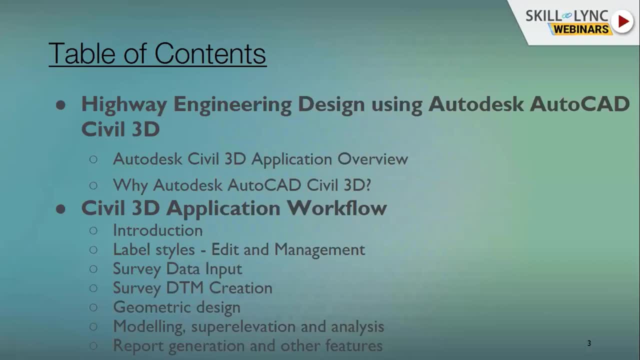 We just chip into the engineering design using the Autodesk Civil 3D software. So I'll be giving the overview of how the application looks like And I would like to tell why we emphasis more to use this application for our projects. What are the advantages? It will be there. 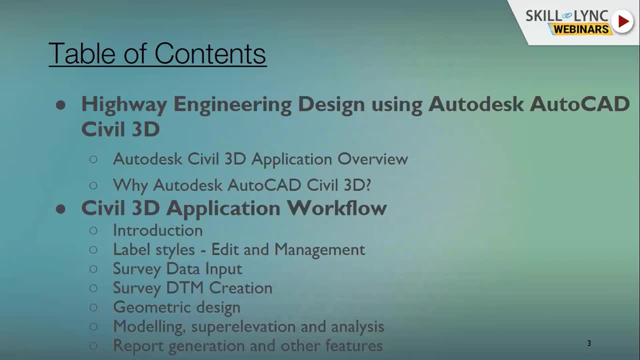 compared to the other competitor applications. So once we have covered that part, I'll get into inner parameters of Civil 3D And then we will also talk about the other features of Civil 3D applications which we will be discussing, about the introductions and its labels and styles, how it will be. 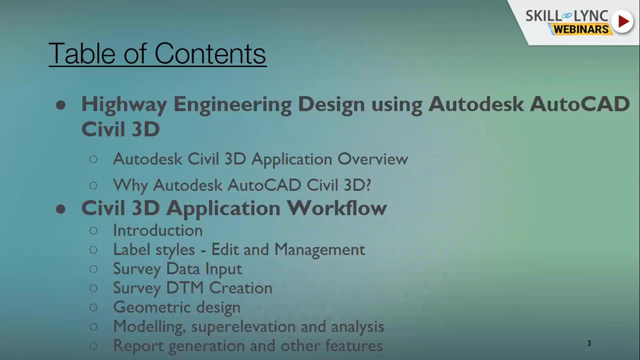 displaying the parameters of highway engineering, Like you all know about the highway plan, highway profile, all the cross-sections, how it will be looking. So how will we control those aspects using these label styles, those parameters? I will just try to brief about. 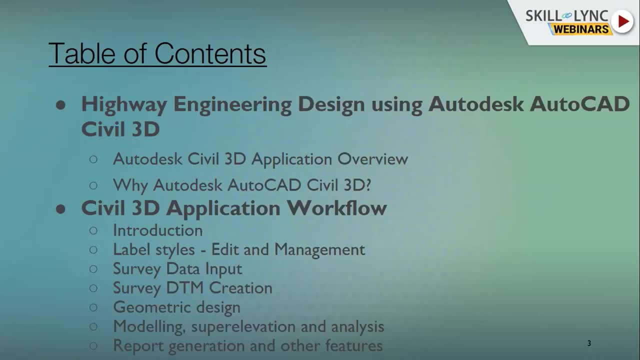 And I will just next. I will be jumping into the survey: data input, How we, from the starting the field, whatever the data we receive, to the design, how we import, what are the different parameters of uh the data will be, the different formats, those i will be trying to brief you and 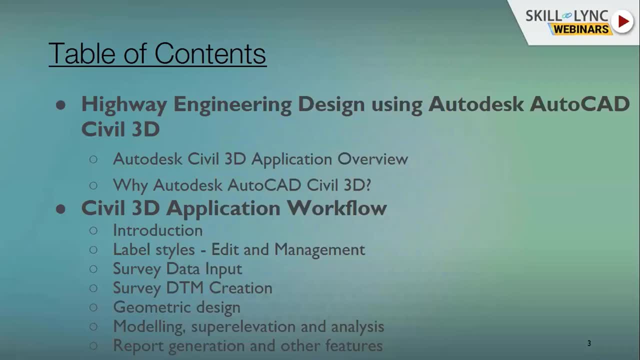 i'll just you know. next step will be the um, the process, the you know template, what you can say of highway design, how it will be carried out, like the dtm creation. next will be the geometric design. after the geometric design, the modeling, how it done, super elevation analysis work: how. 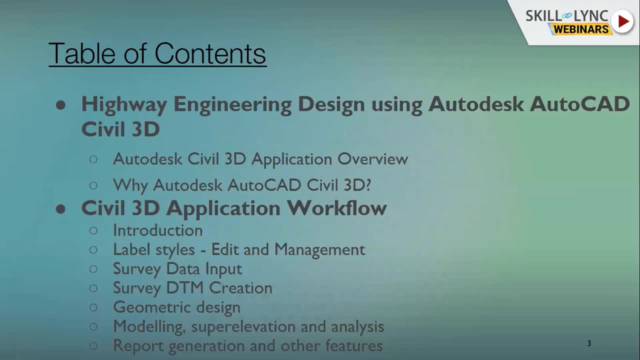 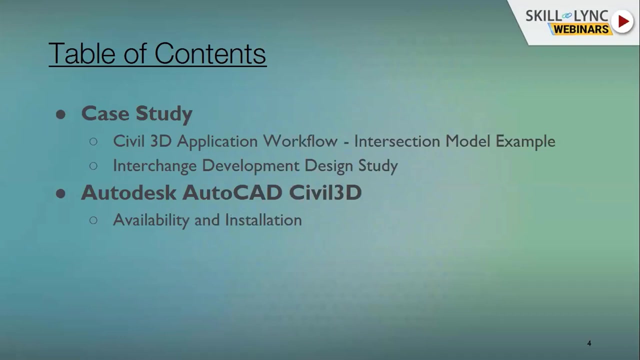 will be calculated. next, finally, the whole report will be generated and also some other important features i would like to share in this uh presentation. so, moving along, i will also explain you about the case study. one typical exam, you know project i would like to share to you, whatever the 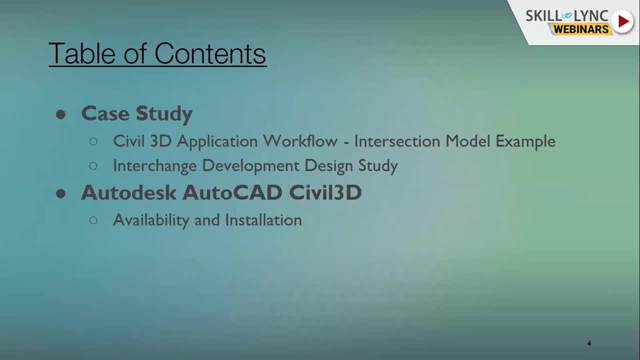 the template. i have just explained how we create the dtm geometric analysis, uh, the corridor modeling. all those factors will be, you know, carried out in a step man, step manner, so that the project will be executed very smoothly and the data, what we receive and what we calculate, what design. 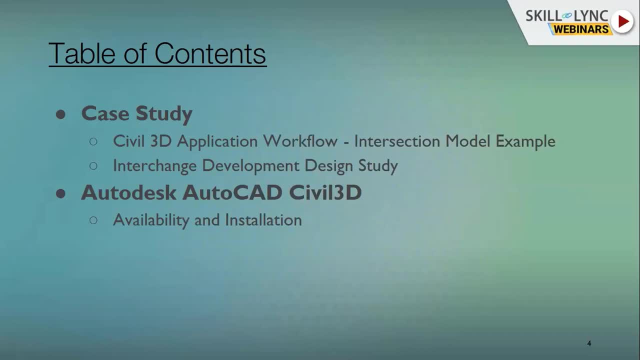 will be, you know, accurately measured and given to the client for this final submission and for, of course, for the construction of the uh site. so here, in this case, i'm i'm using a typical intersect interchange design. where it was a no intersection, it was a junction before. 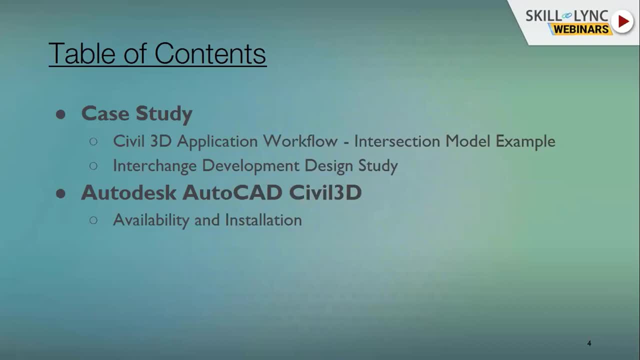 and we are converting into an interchange further. i'll just explain in detail about this case study. so finally, the table intersection in the. in the table of content, what topic will be? there is the autodesk platform. of course, we need to install this uh platform in application, uh application platform to to work with the. 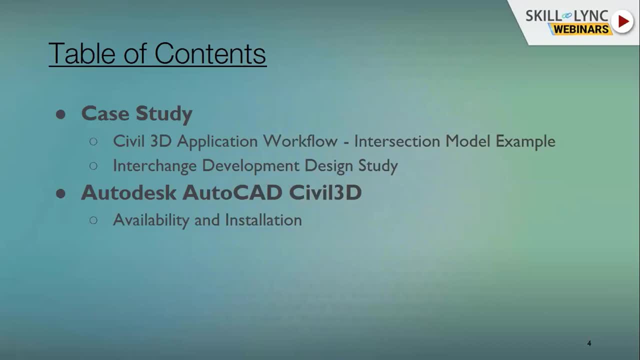 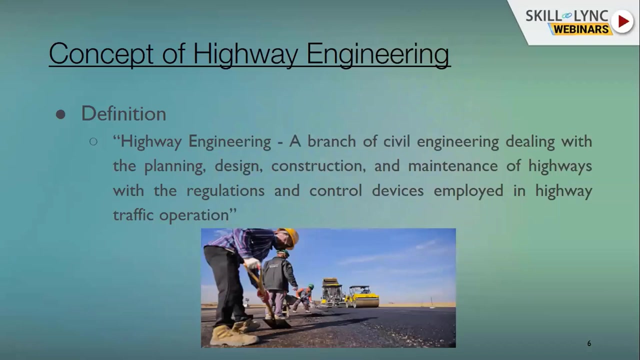 uh, the projects and also where we can approach this one, how. how will be the you know process of that part will be that i will just try to get into the brief about that one. so so we quickly move on to the concept of highway engineering in the prior place. so what is highway? 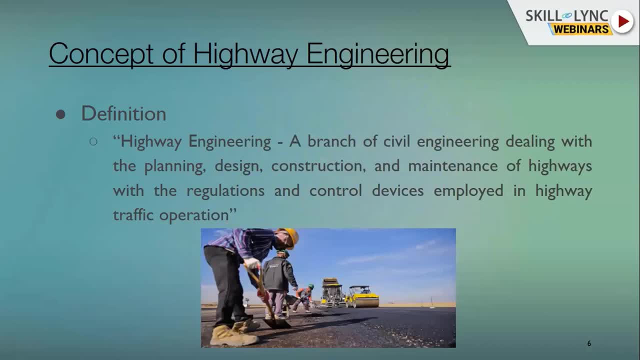 engineering. so the typical basic definition i would like to you know, say to you: the highway engineering is a branch of civil engineering which deals with planning, design, construction and maintenance of highway and its regulations and control devices employed in the highway train traffic operations. so basically, the highway in engineering is about planning, because 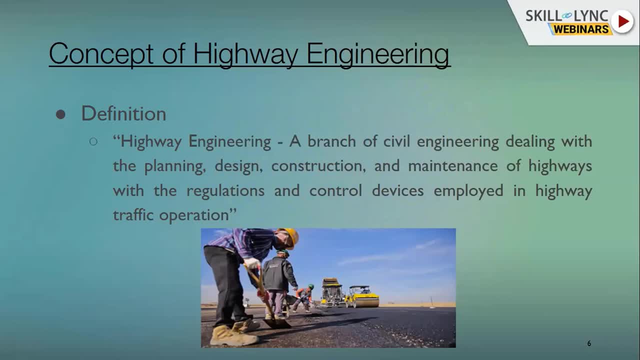 planning in both is a very integral part of the highway engineering. maybe you are constructing a new road or maybe you are, you know, expanding a wide road which is a brownfield, or a field greenfield which is a new, new alignment you are making. so planning is very important part in. 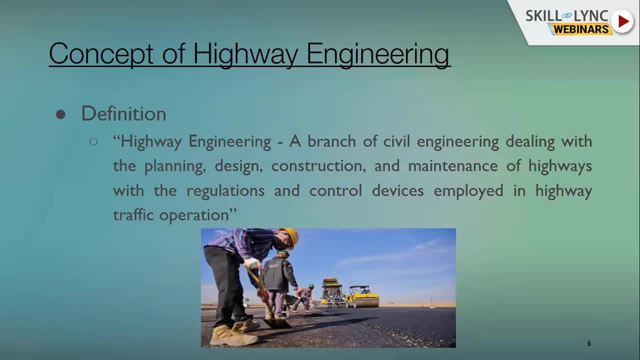 this uh highway engineering, without the proper planning, you can't, you know, do any any further process in this uh field of engineering. so, once this plan is concerned with the client, or with the within the contractor, or within the consultant or the region or the stakeholders, who are all 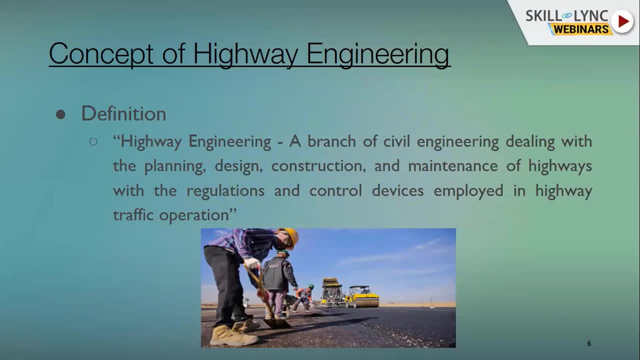 involved. if we come to the conclusion that ss, we need to, you know, construct a road from this point, or we need to widen the road, we need to change an alignment along this road. so all those you know, initial stage is very important for any concrete steps to be taken once that planning is done. 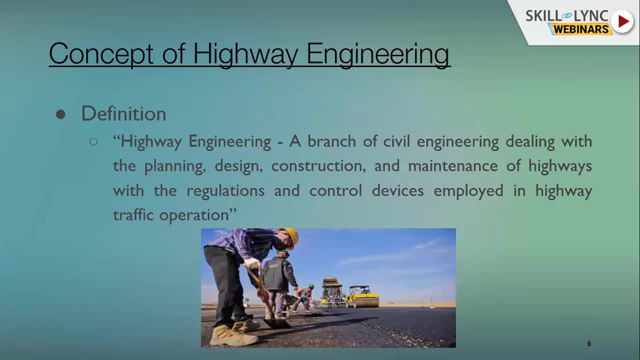 then the next step will be, of course, the design stage, which we think very important parameters in the, in the construction of the highway, engineering, because without any proper design, you will definitely, you know, lose a lot of manpower, a lot of economy, a lot of- uh, a lot of. 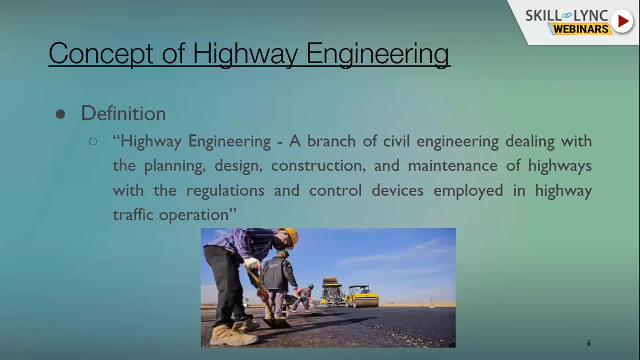 other, you know natural assets as well in the, in the construction of the uh highways, because it involves uh, going onto the field and doing something to the ground there, exactly ground. we need to change the ground. basically i mean to say so for that one we need to be very careful in the design aspect so that proper design. like you, 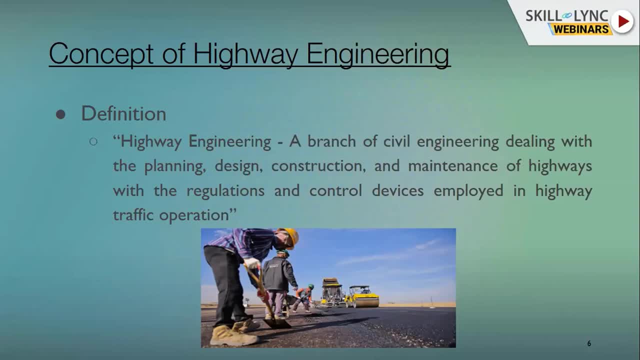 know, filling, uh, or cutting, as an example, i'm saying will be: you know, taken care in the design part, how many, how many earth has to be moved, how many earth has to be filled, uh, how the alignment has to be changed, depending on the design of the road and the construction of the highway engineering. 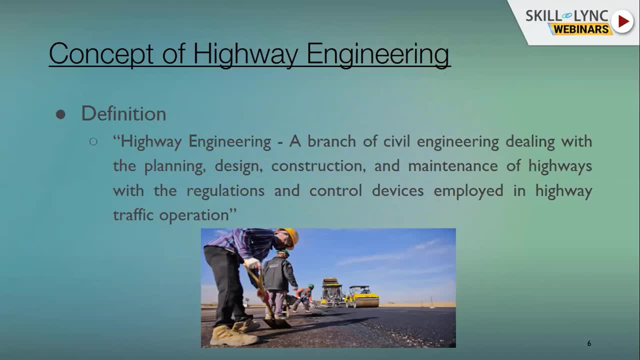 continues without any warrant, of rep quests, getskenning upon the scenario like if you have come across any reserve forest land or any you know lake or pond and monuments. those are the parameters which come along the in between the highway, so we need to manipulate them, or 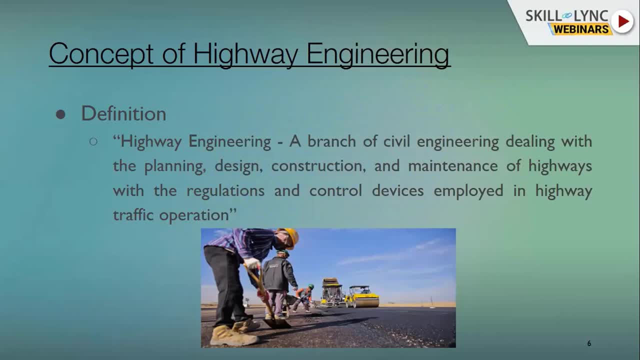 proper, proper respect to those uh factors and we need to try to design that parameter. so designing, planning and designing other very, very basic and very important crucial steps we need to follow in the highway engineering field. of course, when these two has been done, very, very of course it is a physical part of the job, so it will be very easier. I would. 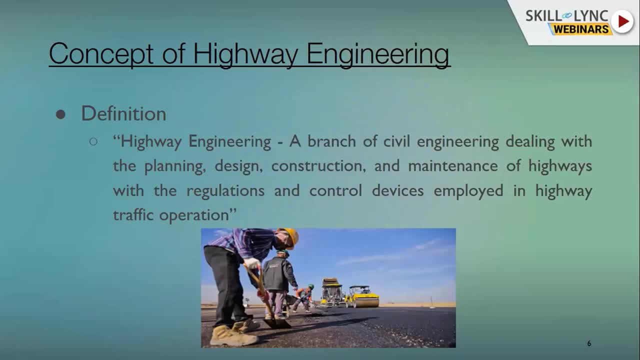 say, if these two parameters has to be properly handled, so then when the construction is done? of course the maintenance is also a very important role, because once the construction is done, if you just leave the road for its way, it will- it will deteriorate in the coming years. 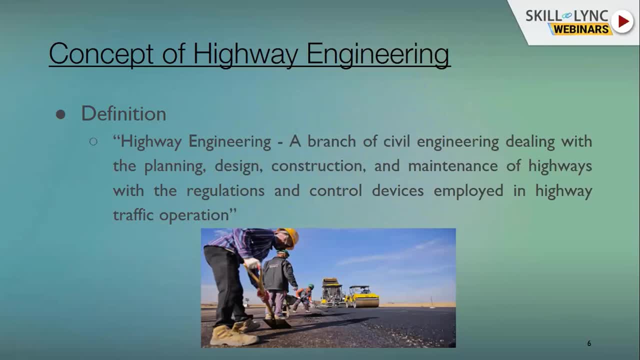 it will definitely lose its strength, stability and its potential for what it is, you know, designed or constructed. so maintenance also will be the important part in the highway engineering. so basically, all this put together, if we need to gel it together to become, to make a highway a very successful unit for the development of the country or or for the 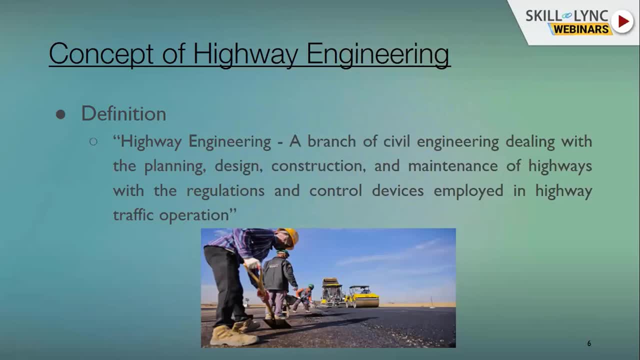 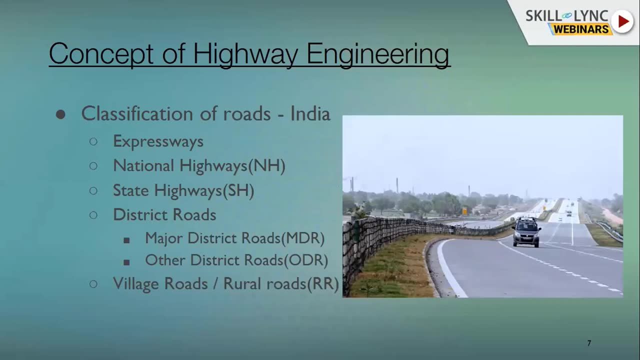 safe. you know, journey of, to and fro, from point a to point b, so that that is very important factors. So the classification of the road. so, coming back to the after the definition, we are not try to touch about the classifications of the roads, so in this case I'm taking a typical. 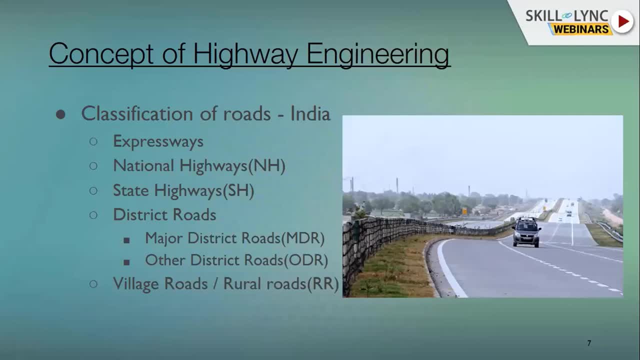 example of India's classification of the roads. so in India, as per the north Ministry of Road and Transport, Highways roads are classified into this format- what you see in the screen- like expressways, national highways, state highways, district roads, which is again bifurcated into 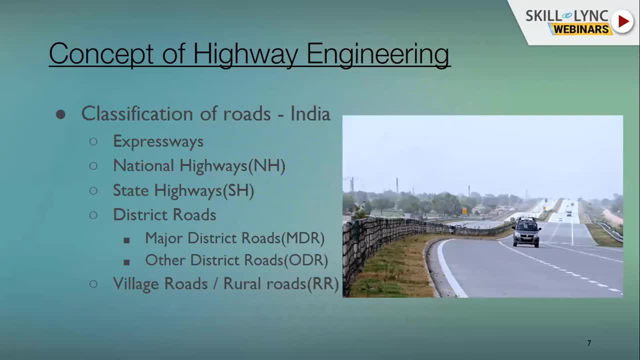 major district roads, other district roads And finally evalators. So these set of roads are being no control by different authorities at different stages. if it is a national highway, it is controlled by the central. the express free also is controlled by the central government. and coming back to the other subcategory of 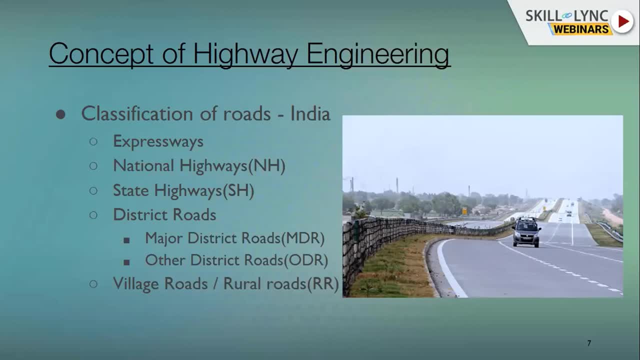 sorts to be controlled, whether the different different departments- So those were- those will be the clients who are handling the whole the sectors of the roads, even from planning to design to maintain 2200 0000, 0000, 0000, 0. 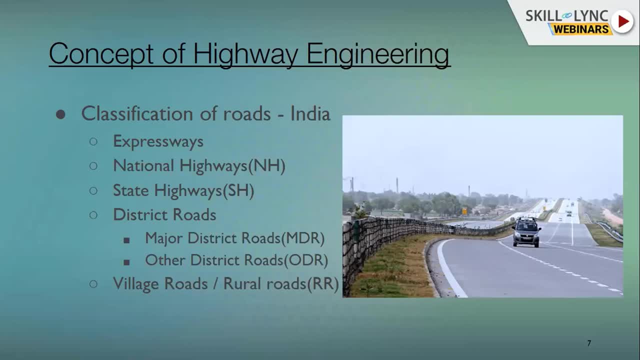 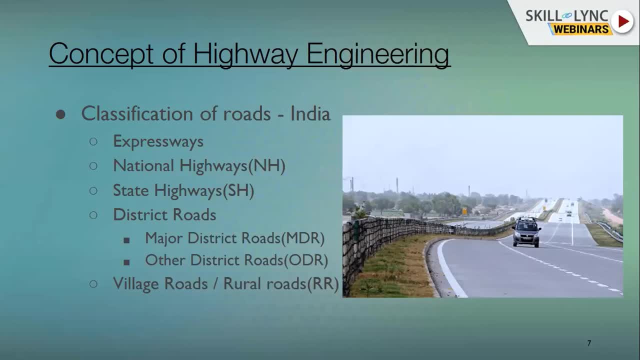 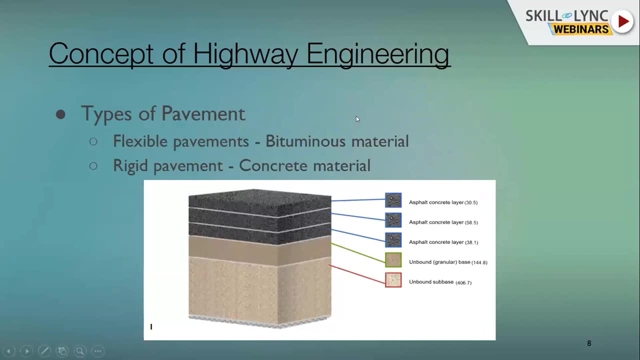 of the roads has different set of codes to be used in this design and design purpose. So next, moving on to the types of payment. So we have, as I said, different classic classifications of the roads. so all the classifications of the roads are broadly classifed into two varieties. 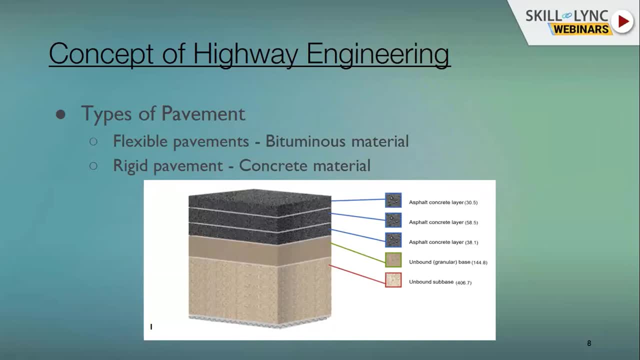 One is flexible payment and one will be the rigid payment. Flexible payment, of course, the materials used will be the bituminous material and the rigid parliament will be, of course, the concrete materials. So these are the broad classifications of the road, that types of materials are used. 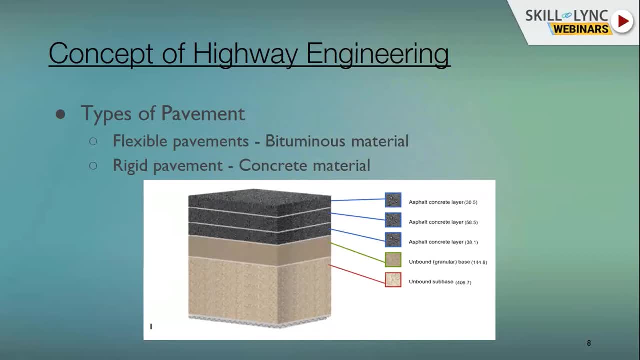 for different kinds of payments. So, depending upon the type of payment, different design of payments are also required Using the different payment question. inaudible question. inaudible codes. The codes are generally, depending upon the country to country, different codes. 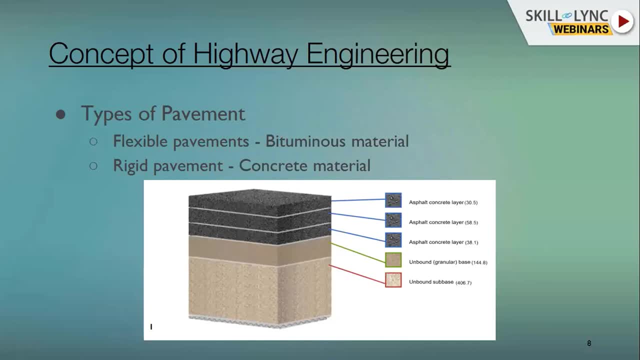 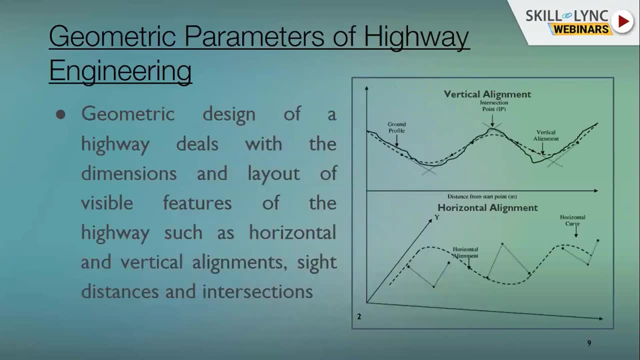 are there. Like in India, we are using the Indian Road Congress as the standard codes for any design and development of highways. So next, coming to the geometric parameters of highway engineering, As I mentioned in the design stage, this will be the crucial. 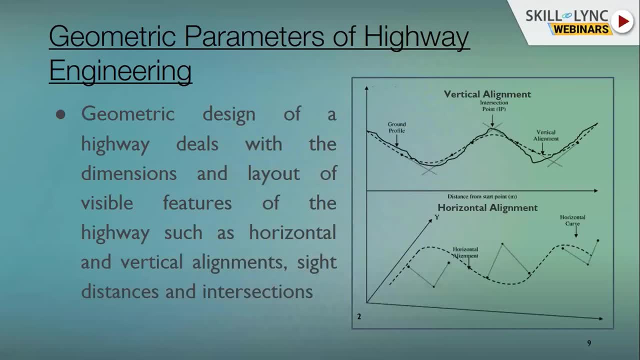 part of any any engineering design. So this will start the template of how the road designs will be taking forward. So first and foremost will be the horizontal design, which is nothing but the collaboration of geometries, I would say like straight go transition, which is 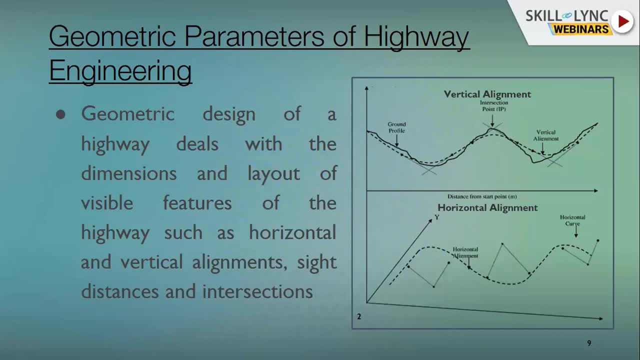 like you know, starting from zero radius to the curve radius. So those are the features, we geometric panels, sections of elements When you be attached together to form an alignment to it. So it may be a straight go and a straight within between the transition, or it may be a straight curve, curve and transition. So 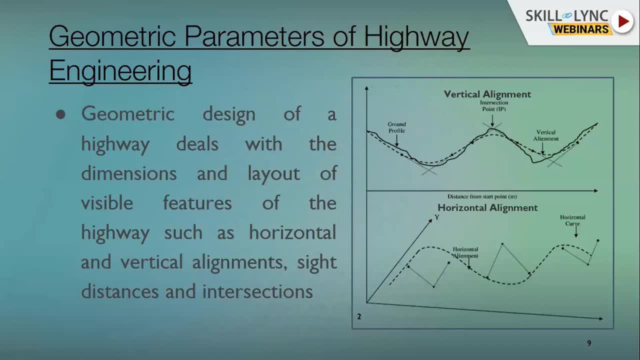 it depends completely on the type of sections we are designing. If you are designing an expressway which has a broader radius and if you are designing a village road or a major district road which has not that much bigger radius, beginning to try to squeeze in 23 radius, 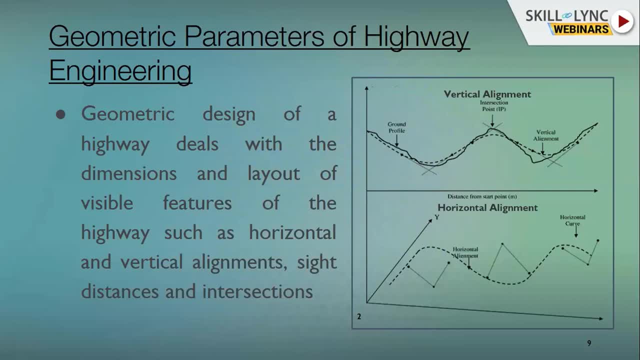 to be, To make it a turn sharp turn. So it purely depends on the classification of the roads what we are designing. in that, all again, we're coming back to the you know codes which we are using. different types of road classification, as I mentioned earlier, has different set. 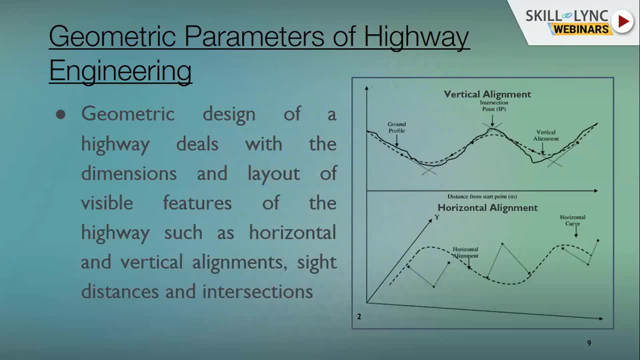 of code values for them. I will show the you know what are the different radius to be used in future further slides So that that comes up to the to the you know joining of these horizontal alignment. we fix these horizontal alignments completely depending upon the two, two kinds, two types of alignments. one will be the greenfield. 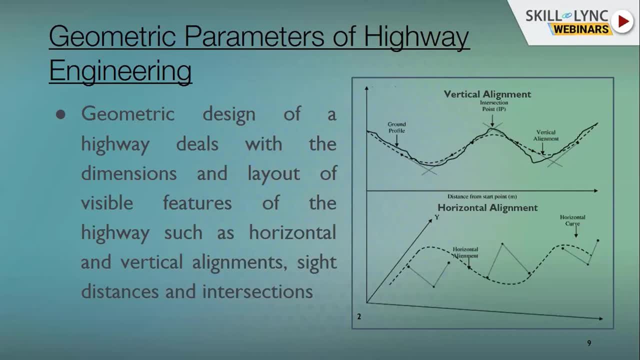 and then one will be the brownfield. The greenfield is a new alignment where we are, you know, giving you know completely a new section from point A to point B, where we try to, you know, avoid all the parameters like roses of forest or a lake or a village coming in. 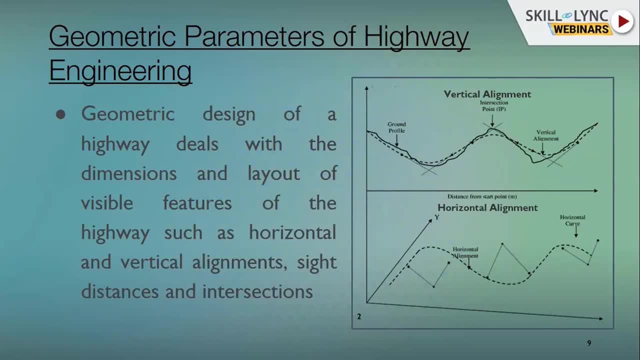 our habitation which is coming across. So those are we will try to avoid in this horizontal alignment. So and we fix the alignment. So similarly we would do it for the vertical section as well. So vertical section is nothing but the cut sections of the horizontal alignment. 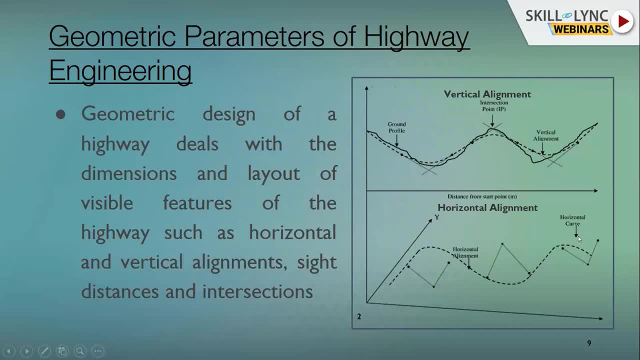 So in this case, you're looking this from the top view And here, in this case, we are looking from the side view. So that that is the difference between those two sections of how we are approaching this section here, also depending upon the types of classification. 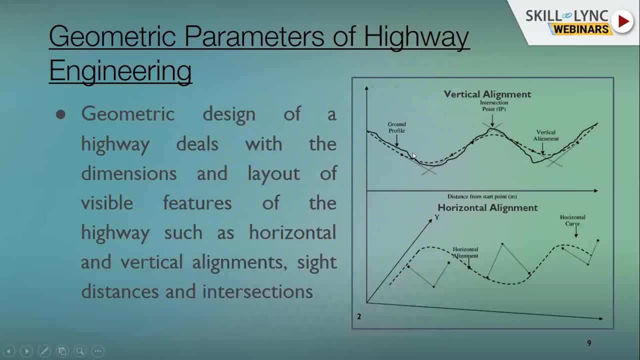 of the road, different grades will be given- Now two straights are called as grades here- which is connected between the curve, which may be a sag curve or a hog curve- Sag curve will be will be to downfall, with connecting to a point which is called sag, and the hog will be the upper gradient and down gradient. 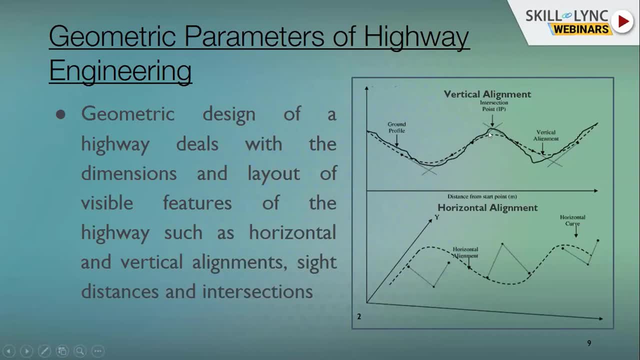 which is meeting, is called hog curve or valley curve. Those kinds of parameters will be used for this design of the curve. Okay, Okay. So vertical alignment. So again, this will be depends on the classification of the road or terrain of the road. I would like to say, if you're designing a vertical place, you 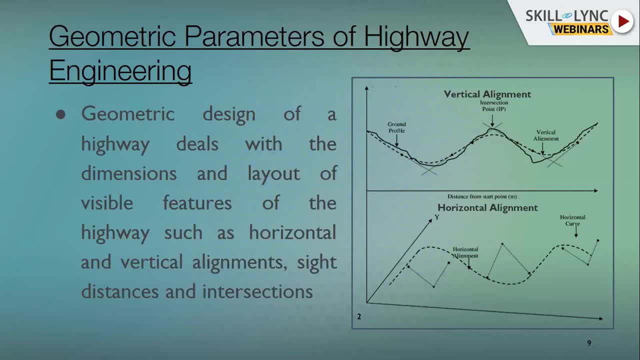 know, you know playing area, that much minimum grade we can give, or if you're designing it in a hilly section, it will be a completely different ballgame. So all those factors will be coming to play in this geometric designs of highway engineering. 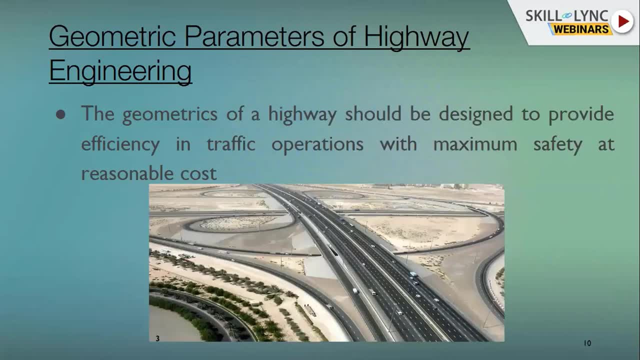 So So why we need to give this geometrics will be important factors, because in it plays a very important role in designing the safety of a traveler on the road, because if you are not giving a proper geometry, the ride will be very, very unpleasant and unsafe for. 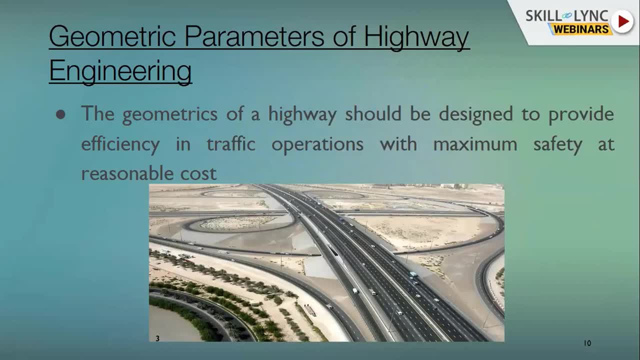 any person who is traveling on the stretch. So to make a person's travel from point A to point B pleasurable, we need to follow all these parameters so that it will be a safe and a non-linger journey in the highways, for redesign and in for the projects. 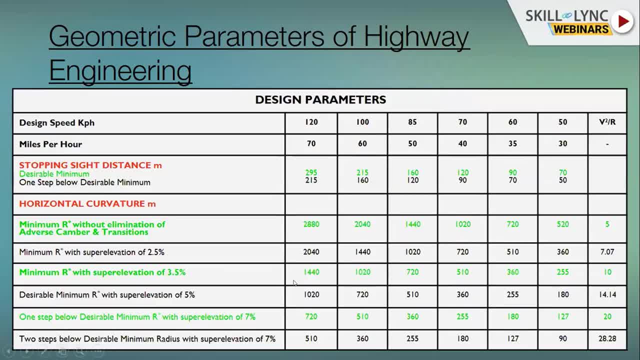 So here is a table I would like to share which is from the UK standards, like all DMRB, which is a design route for roads and bridges: design manual for roads and bridges. I have summarized the what are the important parameters we use for the 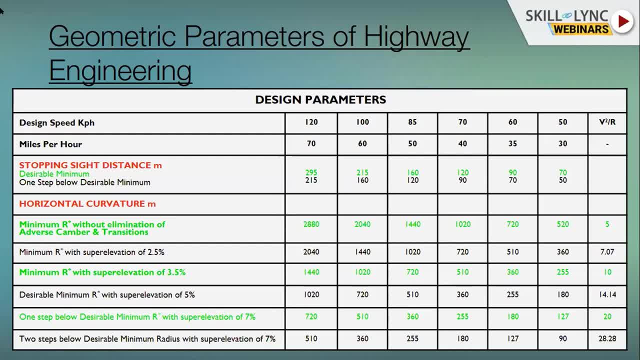 journey geometric design of horizontal as well as the vertical sections. in the left hand column you can see the particulars, what we are trying to issue here, which has the design speed- we have different design speeds here- which is again converted into miles and we have stopping sight distance for that particular design speed and horizontal curvature minimum. what 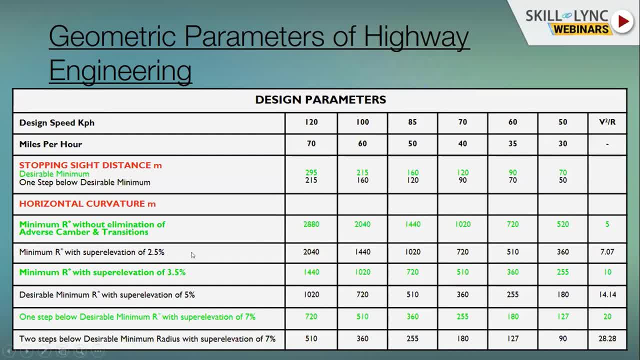 we need to provide for this design speed and once below to the minimum, with the super elevation of particular value. what are the things we need to provide? and again, which is difference of elevation? we can change the curve radius to the into our design aspects. so those are. 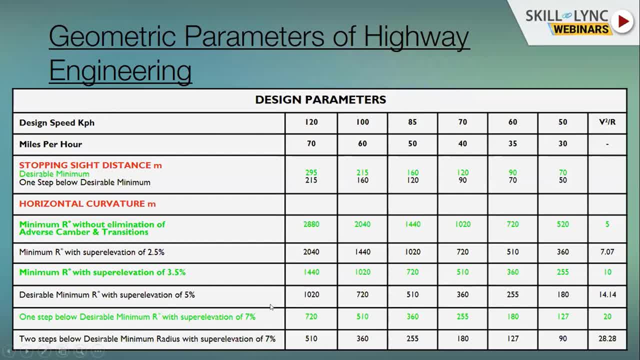 the applications we can use in this parameters. so what we need to try to understand is: we can't memorize all these values in our mind, so what we do is keep a chart in our design table, or the best scenario. what I'm trying to say in this application will be: now we 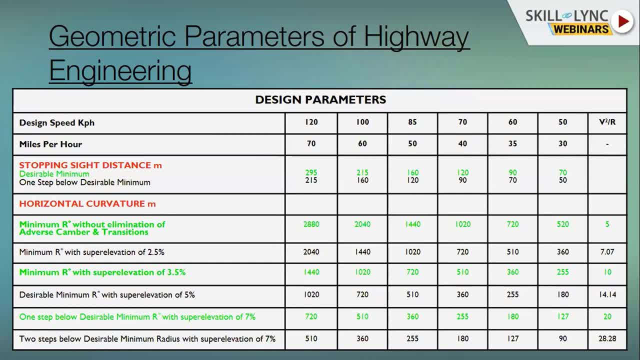 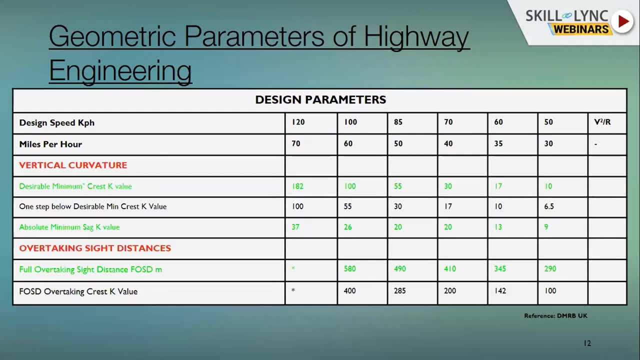 can just feed this value to the design speed. the application takes care, the civil 3d application takes care of this value and it gives a reminder to us if you are deviating from this design values, so that we can optimize this value, design value, and keep this design value standard for our designs as well. so again, this will 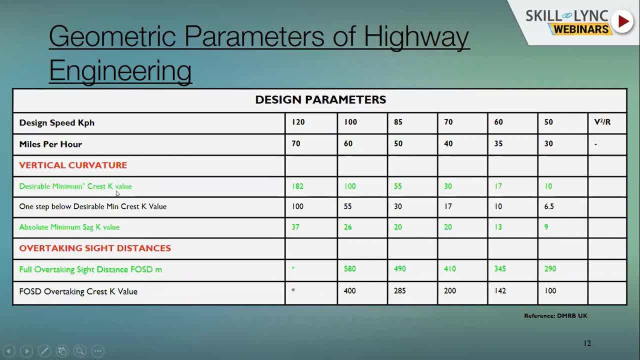 be the vertical parameters. so what we are using, so what will be the KVLK value, is nothing but the geometrical. you know, conversion of two grades and you know to be to be used in that. So what we are going to do is we are going to take the KVLK value and we are going to 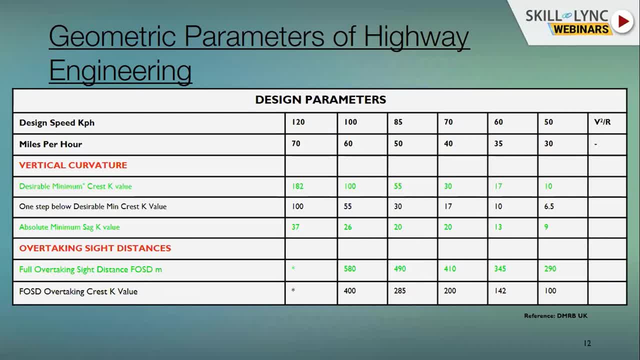 use it directly. instead of the larger value, what we receive in the radius of the vertical curve, we are just converted into the K, the value which is called K, which is constant, so that we will directly use it from the code. so we won't, you know, go back and calculate. 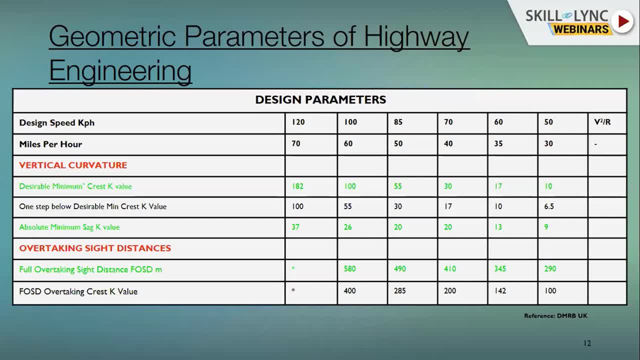 what will be the KVLK in different grades for different and all. so we just take the speed of the road and the grades. what we need to achieve, so what were the K values- would be coming for this particular sag or the hog curve. So those are the direct approach we will be making in the, in the, in the corporate designs. 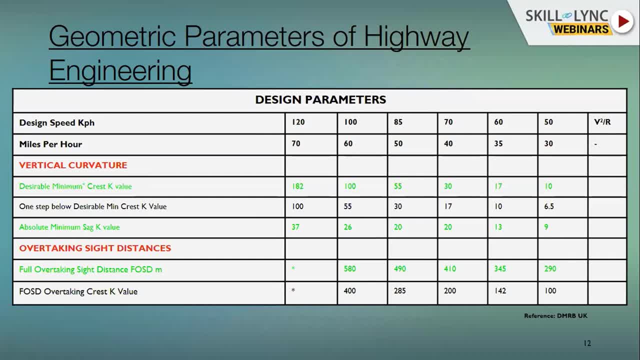 so that it will save a lot of time in the, in the designs, and also we can just, you know, go for the drawing, or you know product drawing, drawing productions, or you know, completing the projects with, with minimum effort and using this course. so these course are very 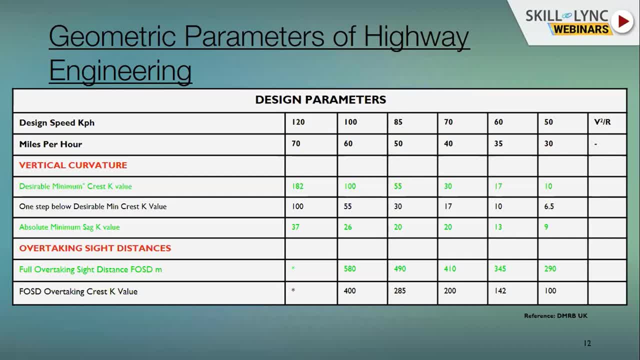 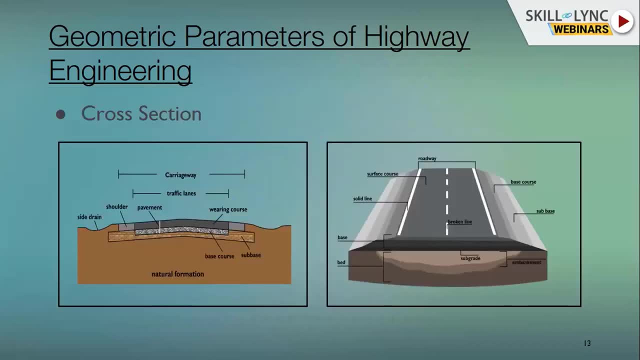 important to follow in the any highway projects. Maybe it is a greenfield project, or maybe it's an improvement of the existing projects that we need to take care in in mind while we are designing the highway, highway engineering projects. so, yeah, so, once the geometry is done and how we are fixed, the horizontal and the 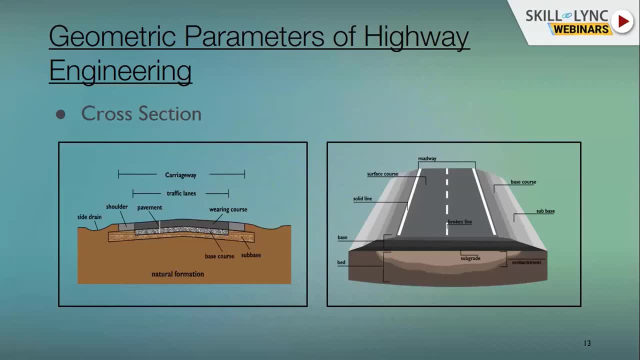 vertical alignment of the road. next comes the important parameters, which is cross sections. so it will be the, you know, body of the road, basically, once we, you know, finalize those aspects of our horizontal handbag, so we need to decide the the type of cross sections for meeting, to provide. 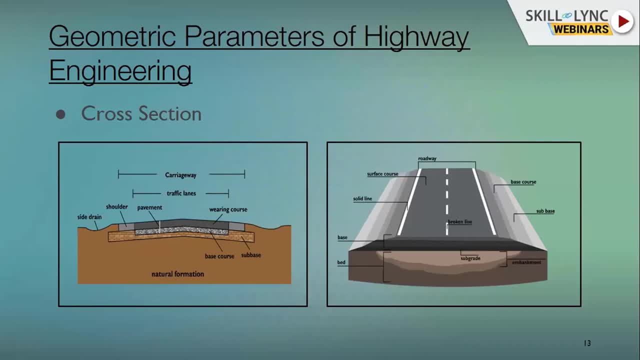 In this, You know, example I'm trying to share, share you the single carriageway cross sections where we are having a typical traffic lanes and different kinds of layers of payments, which which has its own, you know, specifications and importance to be, to be a, to be maintained. 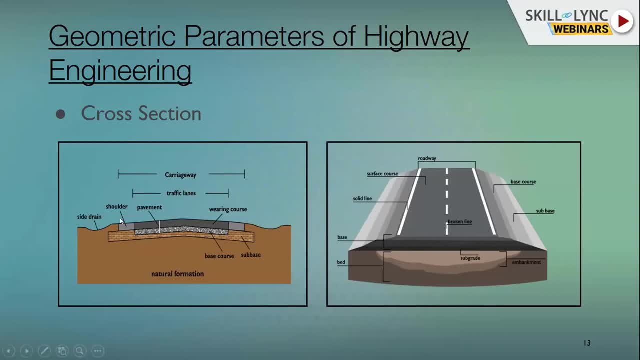 in the highway projects. So, coming back to the, in a carriageway, here it will be, the traffic lanes will be important. The feature of the carriageway, the, the other part, will be the shoulder or the verge, what we call. that also will be place a important road and a side drain which we need to provide. 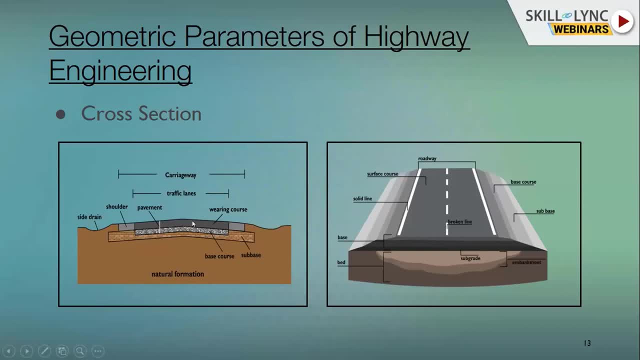 to collect the water whatever falls onto the traffic lanes that has to be brought in. this one below will be the payment layers: sub base, subgrade course will be the base formation and the sub base base and the varying course. so the all this, not different layers of payments. 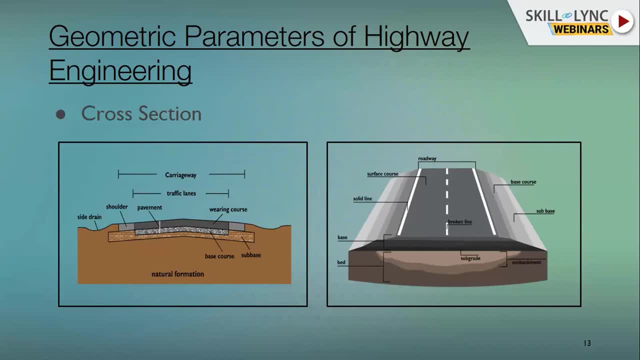 have been provided for the concrete road. Every other concrete road it will be a different scenario to be maintained. so, depending upon the type of payment we use, and and, and then the parameters we use, we decide the cross sections with various, various factors. So this is one such basic example I would like to show once we're done with the horizontal. 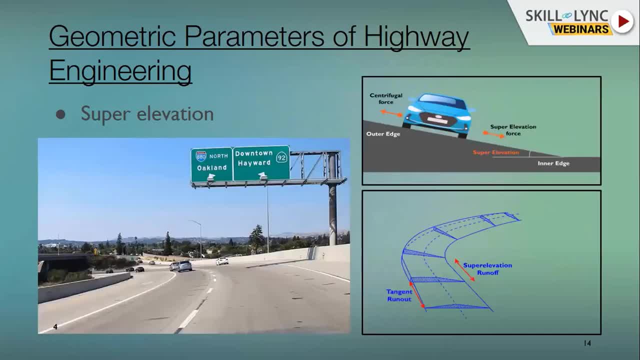 and vertical. We go for the cross sections design and construction. in the cross section design we just come across different analysis Which put forward forward with a couple of analysis, our main analysis, what we do, i would like to show display in this presentation. the first and foremost will be super elevation. um many of you have been aware. 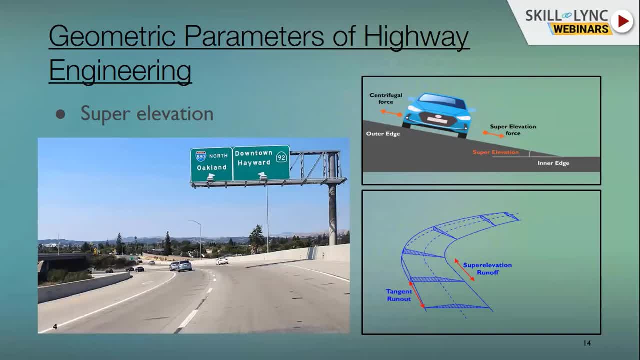 of you know, you know, traveling in the, in the road, uh, experience this kind of, you know, force. while we are not going on a horizontal curve, you may be experiencing a pulling force which is, you know, pulling you from from, away from the road, actually to these sideward directions, so that that force 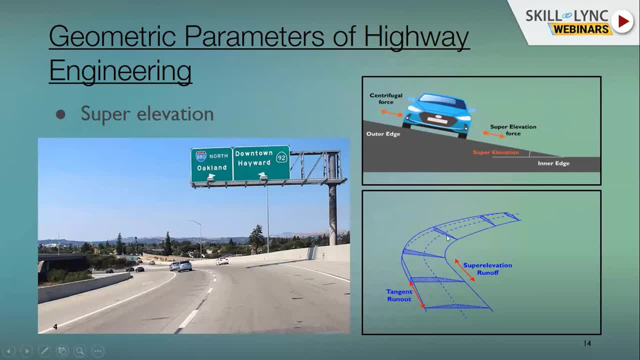 is called a centrifugal force, which is pulling away from you, from the center, because of the drag which we are experiencing, while we, you know, covering this section. to avoid this- you know force and make the- uh, you know- journey along the curve smoother, we provide a concept called 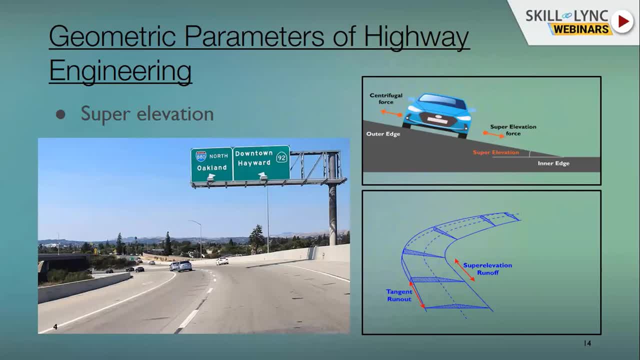 super elevation, where we will try to raise the outer edge a bit higher from the inner edge. that also depends upon the various uh parameters. i'm not going to detail about that parameter. so you, depending upon those code values, we will just raise the the outer edge of the carriageway a. 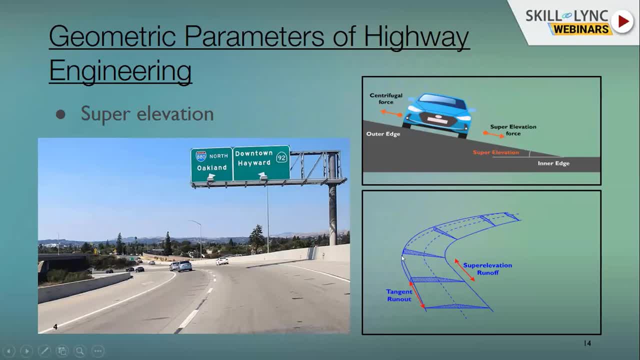 little bit, as you can see in this image, where we raised the outer edge a little bit, so that the inner edge will be at the same level of the road, but the outer edge will be a little bit higher. so so once we travel along this road, that force will be, you know, minimized or 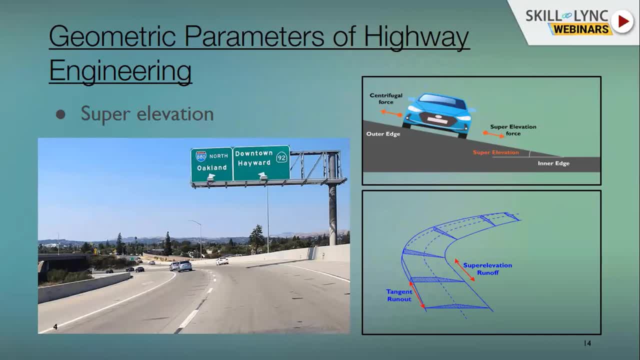 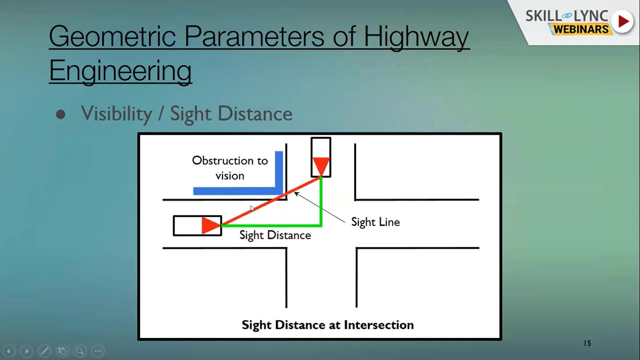 countered so that uh not traveling will be easier. so that's the concept of super elevation. all those values will be taken from the course again to to achieve this uh, super elevation. the next one more uh parameter of road safety precautions will be visibility, or the site distance. uh. so in this, uh, in this slide, in what image you are saying will be the junction? 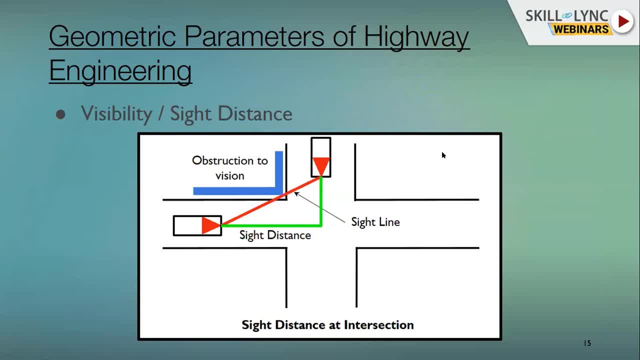 visibility, um, what we need to achieve so. so it's a if it's a you know typical case and you know tricky situation where we are seeing this unprocessed left over side danger lane vendor, so we want to have all of those parameters and with that we will wrap up the verbal instructor. 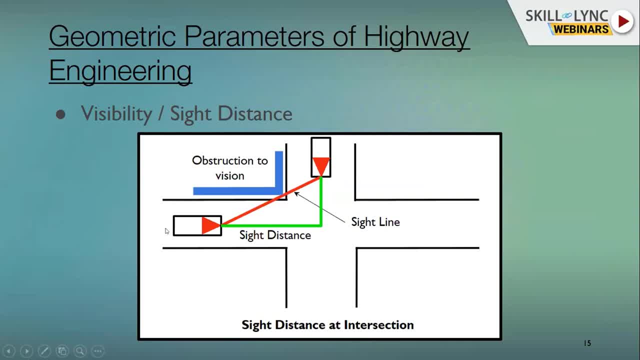 we don't have any traffic light to control these junctions And if you are traveling on this junction and you are not know how the visibility of the other road vehicles which are coming, So at this point it will be very important to give the minimum sight. 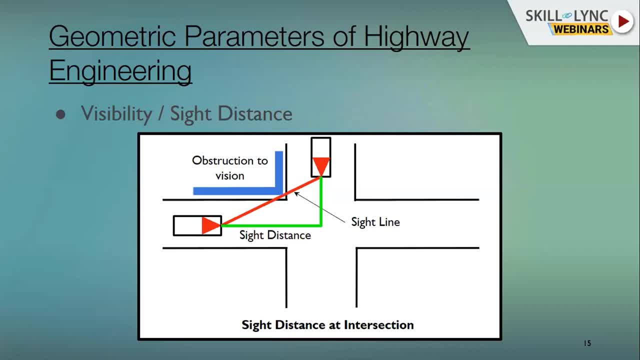 distance, distance length for any particular junction design and also the obstruction vision. So this vision, which is called as a visibility is play line, what we call, should be minimum so that the vehicles can- vehicle driver can see what's the other roads. Is there any vehicles? 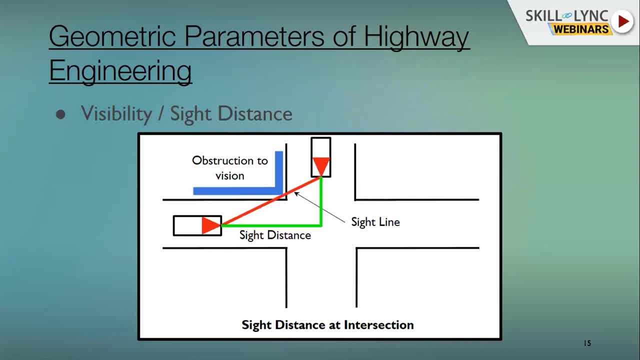 coming along the roads or not. So again, this distance depending upon the type of junction, type of carriageways. all these parameters will include designing this distance as well as the visibility displayed, their distance. So that all been provided in the. I'm just trying to explain the concept about it. So we need to provide a certain distance and 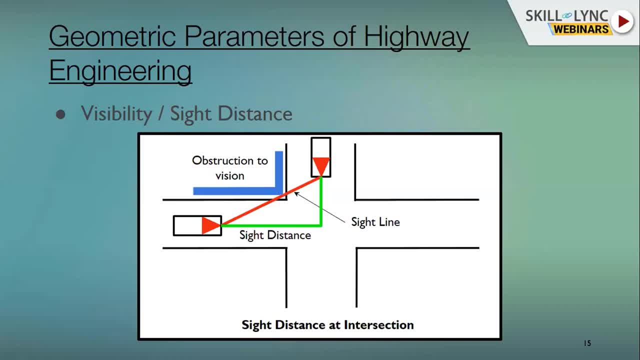 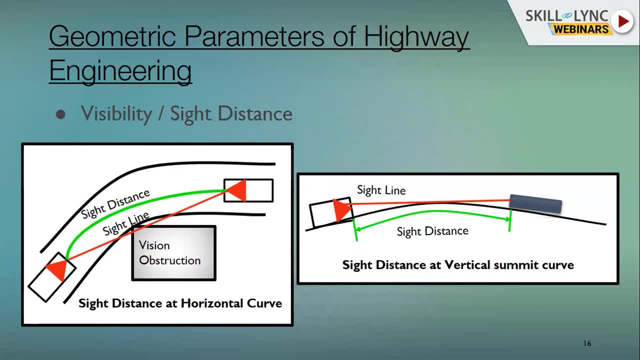 visibility is play length to maintain the standard of the vehicle, The intersection design. So again in this case, in this slide we can see The sight distance, what we need to provide in the horizontal curve as well as the vertical curve. So these are the two other factors where visibility will be tricky situation. so we need to provide. 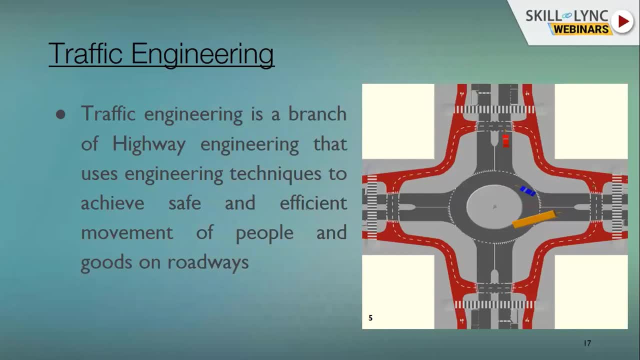 that. So next we'll be moving along the traffic engineering. so traffic engineering is one big factors apart from the geometric design, And I'm going to explain. So traffic engineering is nothing but you know deciding factors of many individual things in the highway projects, like, for example, How we decide the 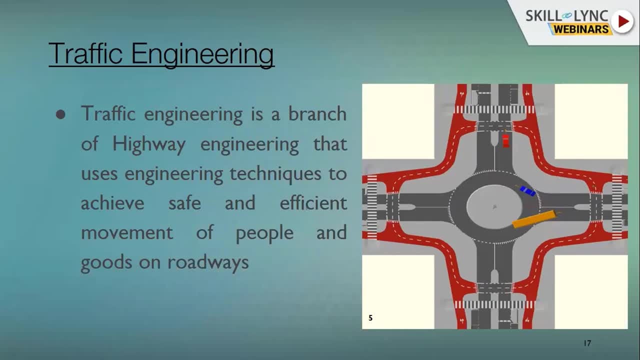 Did the carriageway width what how much lane we required for a particular stretch? that's calculated using traffic engineering. How we decide: is the junction require a signalized junction, or we can control the junction using the traffic signs or road markings. or you need an interchange or you need a roundabout. 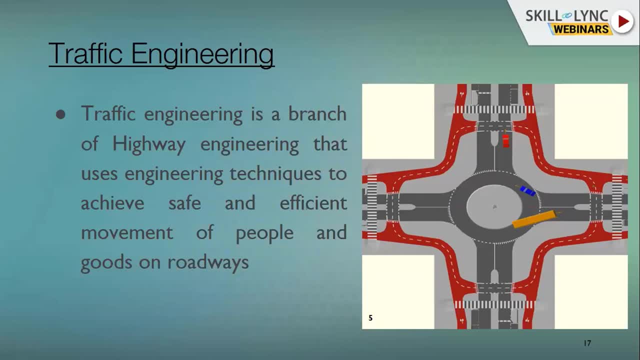 All these factors are decided by traffic engineering. so it is a very important branch of engineering where we use all these techniques to, you know, decide the parameters of the road or intersections, so that the calculation is very important. So for doing the highway design part as well, 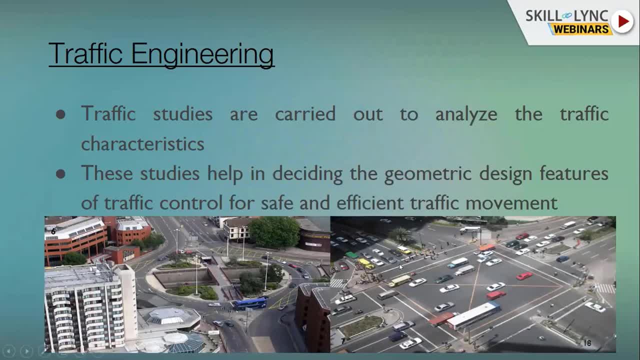 So I'm just briefing about those parameters. so, as I was saying, traffic engineering is very important for you know, doing all those deciding factors in highway engineering. so how it will be Done, though, the factors will be, you know, analyzing the traffic, the volume counts, the origin, destination, 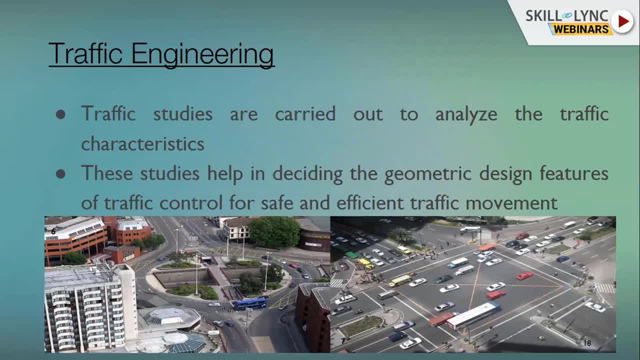 service. so intersection, you know vehicle arc counts. so all those parameters are very important because particularly in junctions, in city roads, at junctions there will be, you know, multiple stuff will be happening at the same time, because the people are walking through the roads and vehicular movements will be there. so it will be very important to decide. 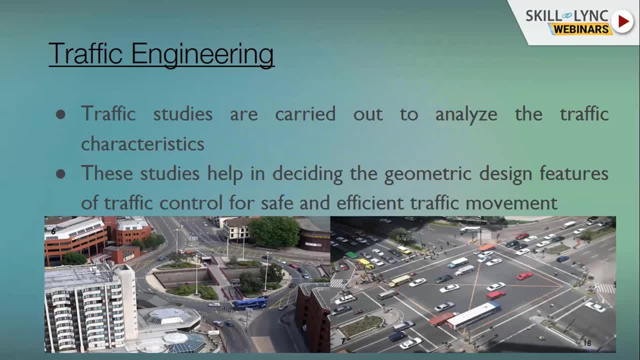 what kind of Junction and junction design we need to make. either we need to go for a signalized junction, or it requires an interchange or a roundabout, or, you know, simple road markings or road signs will control those parameters. so all these factors again will be deciding on this traffic. 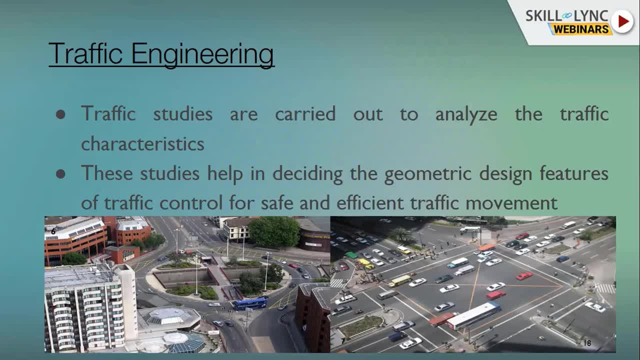 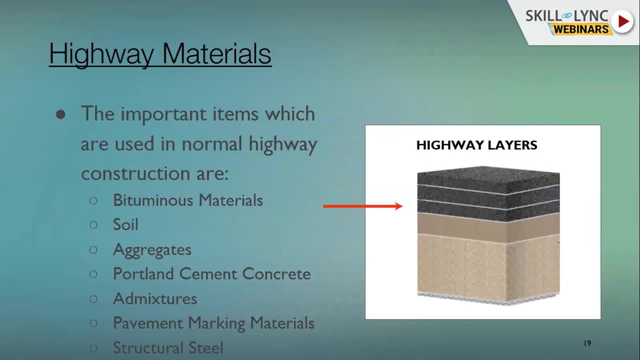 analysis and characteristics. so that comes with a very important role for highway projects. So we have all the parameters, design and all, So next will be the construction. so construction, what we required is materials, of course. so so, as I was saying, different, two types of 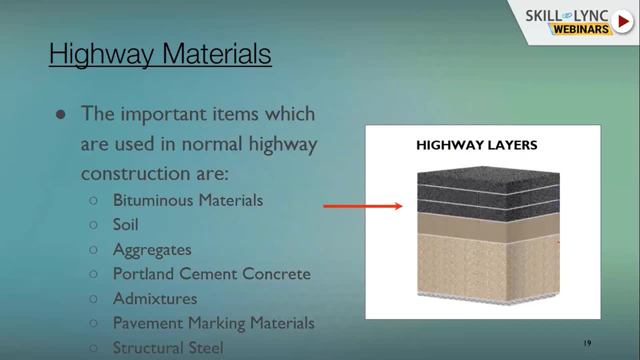 Pavements we have to construct in a particular road sections. for that we require all these basic materials like bituminous materials, soil aggregates, PCC Or admixtures, pavement materials, structural steels. all those materials are very, very important to get into the construction of. 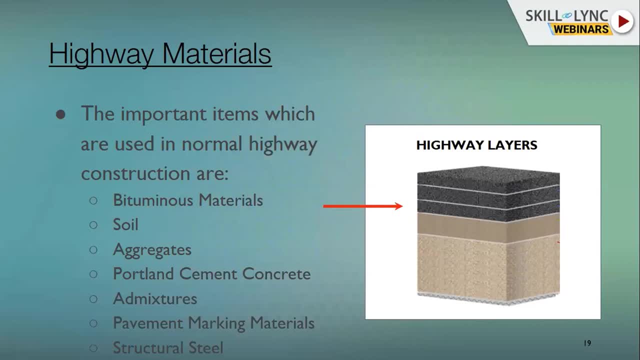 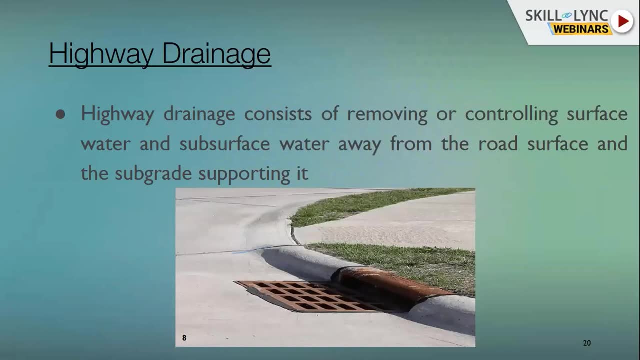 A Roads, so that brief I would like to show to you. the next comes the highway drainage. this is one important factors for maintenance aspect. so So it says that, like, biggest enemy of a bituminous, bituminous material is water. so as soon as 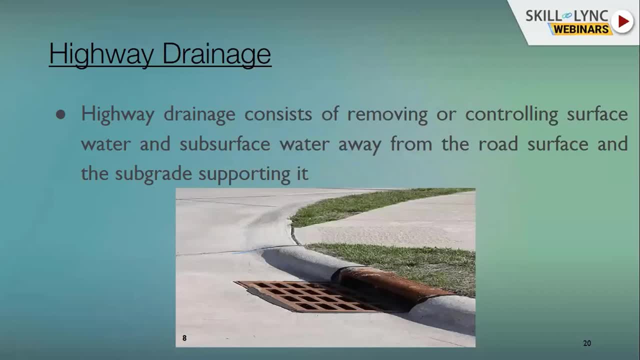 the water comes along, comes in contact with the bituminous. we need to drain the water as soon as possible. so the There are multiple ways to do it. one is, you know, giving giving the cross slope Along the along the you know section of the road, so that cross slope we can just do. 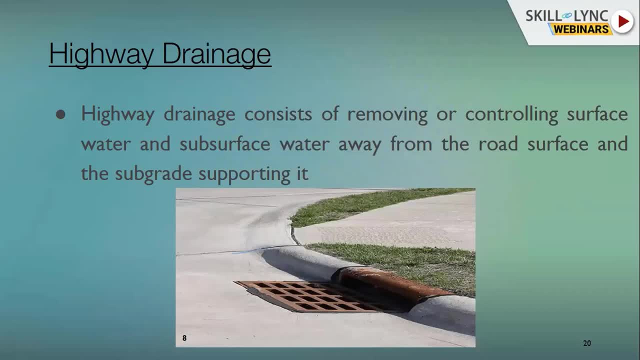 I don't drain of those waters and collect them in the, in the drains at the edge of the carriageway. or you can give the Cross cross drain along the section of the roads, depending upon the No six, depending upon the scenario of the roads. if it is in a different sections, we can just. 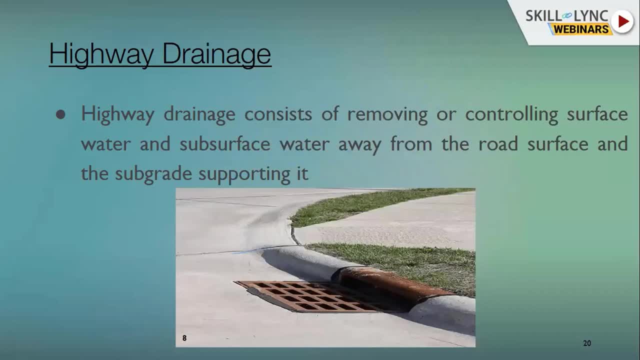 do that one as well. Or build a culvert at regular intervals or a small bridge. minor business end up in a structure Aspects also. we can do give and drain of the water as soon as possible so that we need to take care. well, you know designing the parameters as well. 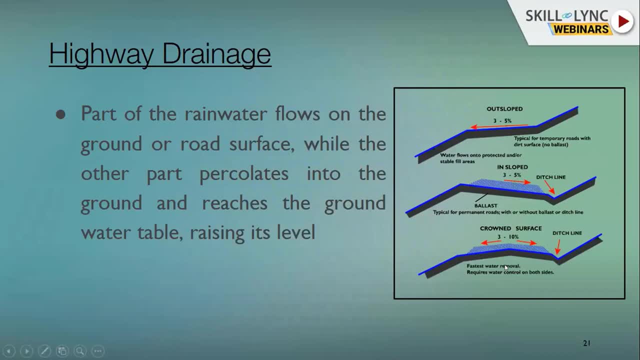 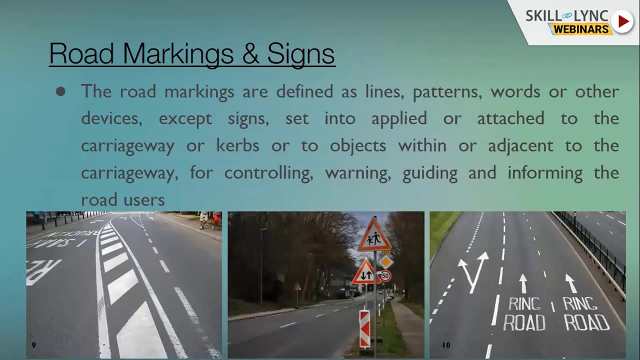 So this will be the you know, as images shows here You can see there are different ways of no moving out, of taking the water out from the carriages, From the road. Okay, So next important parameters will be road markings and signs. So these are, you know, very, very important features for the road users and for a safety. 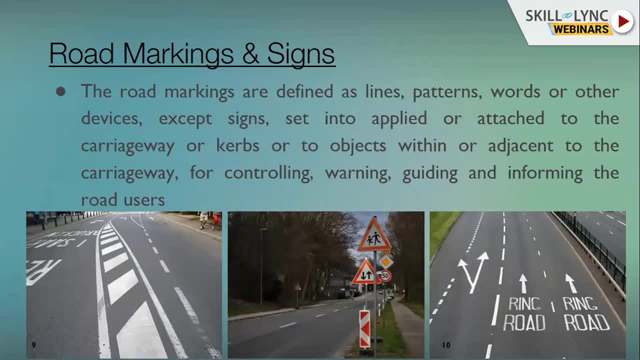 as well as the other pedestrian safety as well. so it gives it shows, multipurpose, like you know. it gives the- you know the road users is control over the road and it says where to place and place him in the, in the, in the carriageway, so where the direction will be. 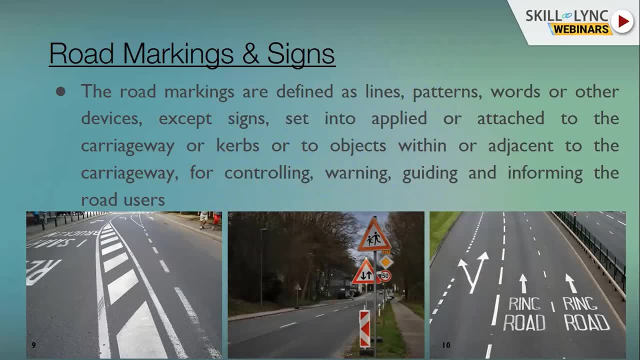 where it is. So these are some of the things that we need to keep in mind when we are taking it: where we need to stop or we need to take the left or the right turn, or where we need to maintain within the lanes. So those are the parameters which controls the road users or the pedestrians will be. 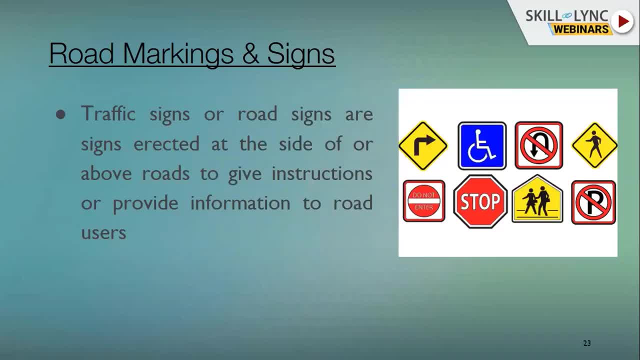 road marking and road signs, So we need to give importance to those parameters as well. So these are some road signs which controls mainly in the intersection or in the high speed highway. We need to provide this one in at regular intervals so that you know. 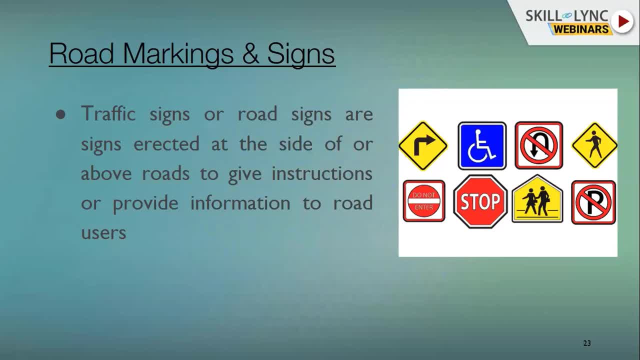 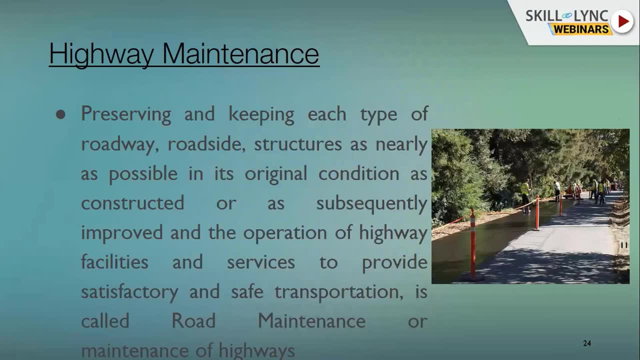 It helps in road safety as well, as you know, guidance for the road users. So, once we have all these parameters, road maintenance and the very important factors which controls the highway project as well, because once we construct the road, preserving and keeping each type of roadways, roadside structures as nearly as possible to its original, 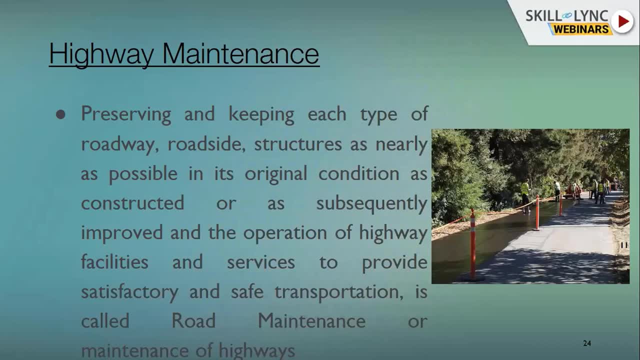 conditions as constructed. so that will be the ultimate aim, But It can't be achieved for 100%. but subsequent improvement and operation, highway facilities and a service to be provided, satisfactory and safe transport is called road maintenance. So basically, we will try to achieve to close as possible to the original condition, regular. 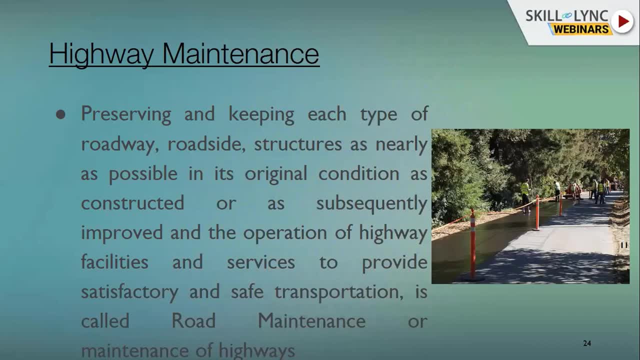 maintenance of the road. In some cases the earthwork maybe just slips off from the road sections because of heavy rain or, you know, substandard construction. So for that one, quick and quickly, you know reconstruction will be very much important. So that's it. 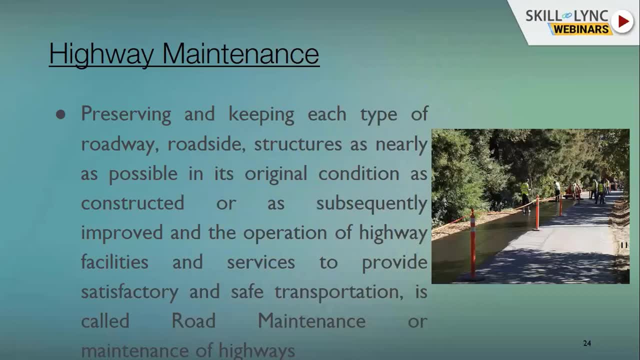 Thank you. So in some cases the it creates a pothole in a section. So once the portal is created, if rainwater is collected there, it will be starting the water circulating through through the, through the road layers, and it will create damages to the road. 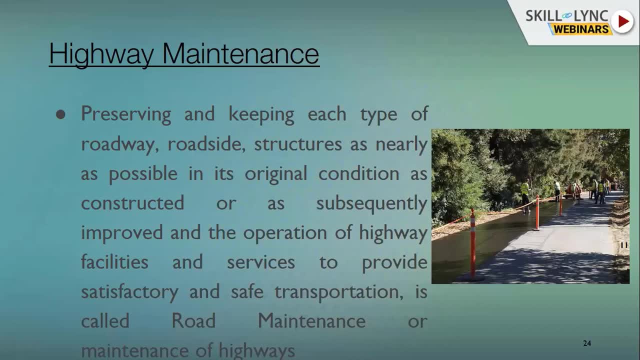 So quick maintenance will be helpful in the long run, for the long run of any heavy projects. So maintenance will be a very crucial part and also it improves the economy as well, because construction takes a lot of capital to be invested for a particular stretch. So maintenance will be, you know, if we maintain the road properly, that capital can be you. 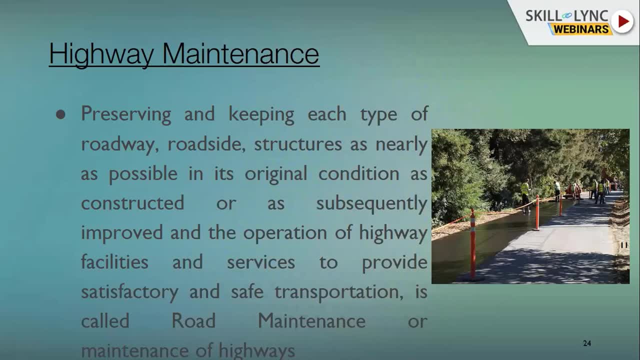 know, stopped into going into that road for any reconstruction again and again. So once we construct, we construct it with thorough planning, design and analysis and proper- you know, with proper- construction material. once we do that, we try to maintain that one for a particular stretch. Thank you. 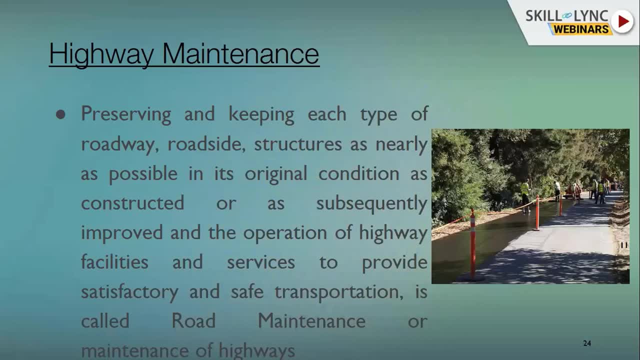 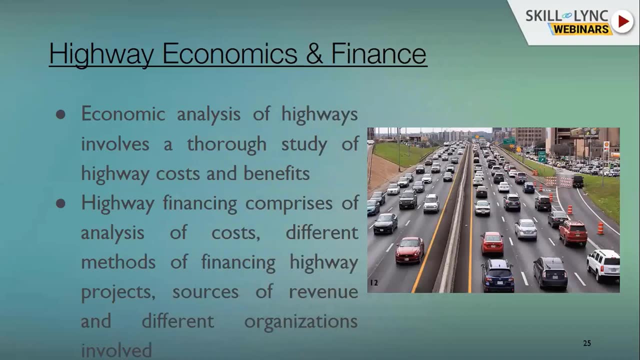 So that will lead to a good practice for any heavy projects. So what I was trying to say: once we have all these parameters, rebuild what it gives, final output of the roads will be, of course, due to give the- you know, the country, the region, a better economy, because connecting road connectivity is very, very important for any any growth. 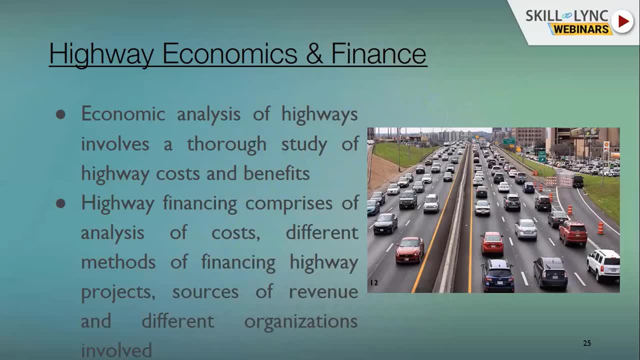 of the countries. without you know, proper connection, It will be very difficult for any country to to, to develop in the, in the, in the pace what we, what we, you know seeing through. so proper infrastructure is a, is a very much important because people use this road to to reach their place and do their business or do the no economic their their bit. 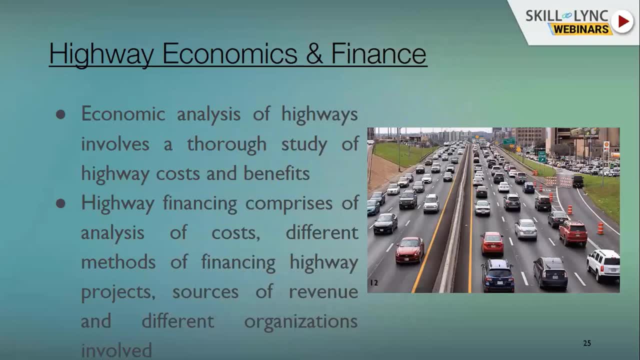 So we as a engineers, try to give them as safe and as quick mobility as possible to reach their destination and do their part of work. Thank you That that that improves a lot, because if everyone communicates with a safe and a quick manner to and fro, it definitely helps a lot of time. as we experience in our countries, the city roads are not jam. 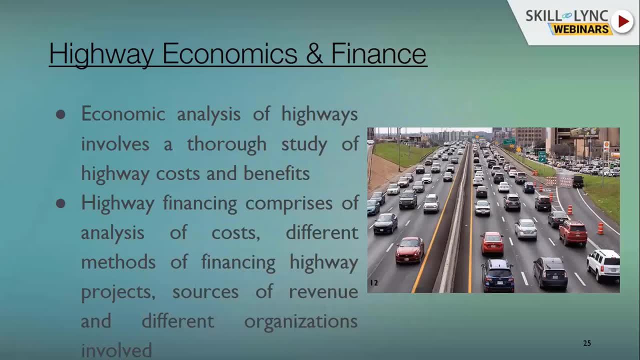 packed and we stuck in traffic for many, many hours, so that if we avoid that one, it gives people to reach their places- maybe it's a personal place, or maybe it's a professional place- and raise them quickly instead of Staying On the road. that will be leading to the economic improvement, as well as the financial growth, of individual. 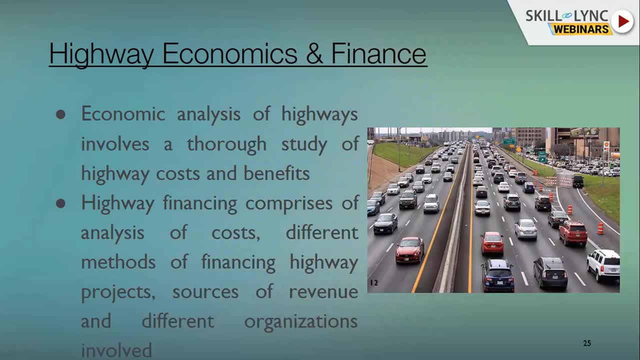 aren't, as well as the countries growth, so that's how it plays a very important role on what we are trying to achieve here. so these, these are the- with that being said, these are the parameters of highway engineering, starting from planning, designing, analysis, maintenance, as well as the final output of, you know, building. then, 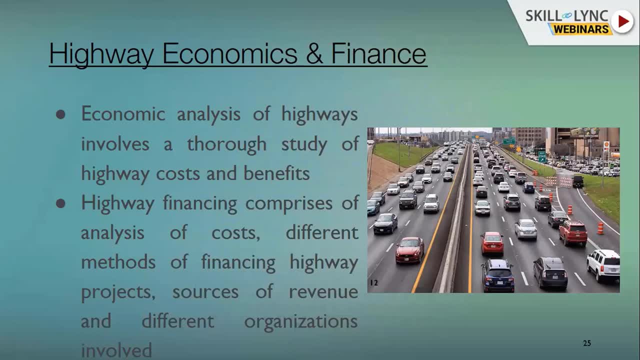 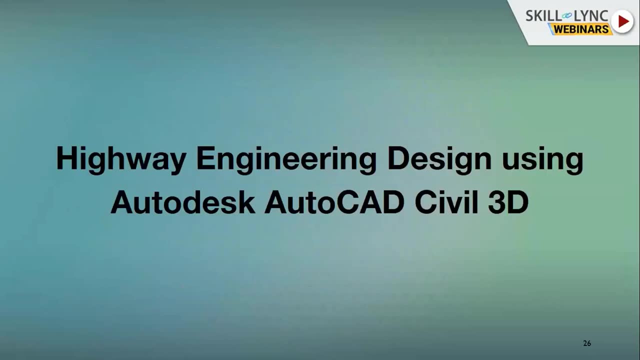 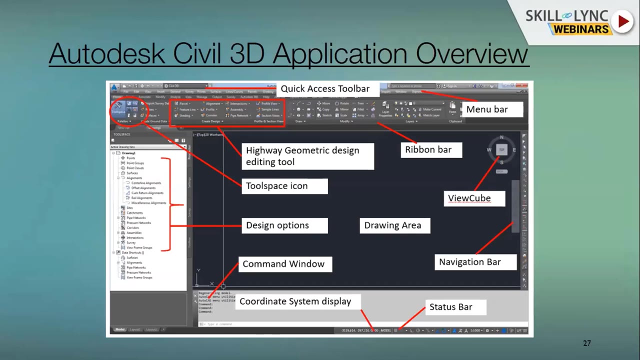 economy. so these, these are the basic about how engineering. so we quickly move on to the other topic of today's webinar, which is designing a highway engineering project using the Autodesk civil 3D. so I'll quickly walk through the civil 3D over you. so once you open the civil 3D application. so every year the civil 3D has 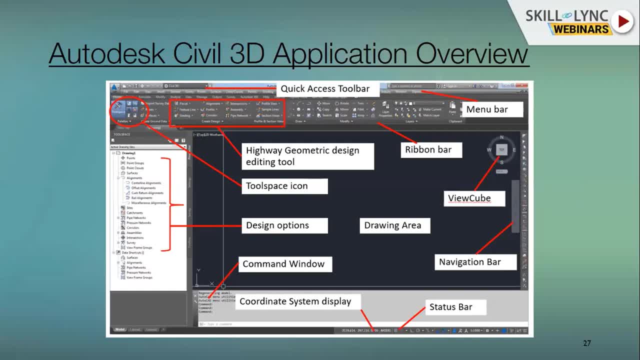 different versions to it. so this is the version which I a, which we are using, like in two thousand 19 version. So this is the you know parameters which you come across, that and then once we open this one. so I'll just try to explain. 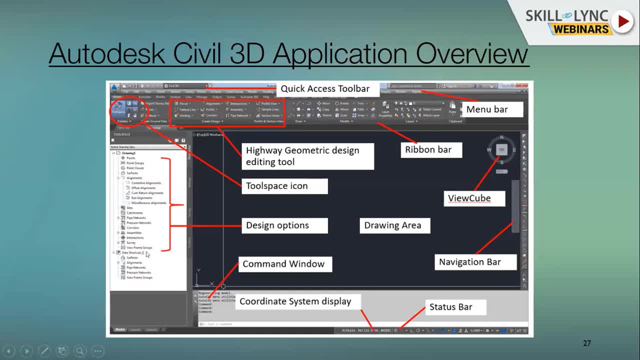 what are the important factors we need to take care while once we have no open this applications? so what is our civil 3D? so civil 3D is a design applications which works on the background. off I took. I took it, so it has all the. 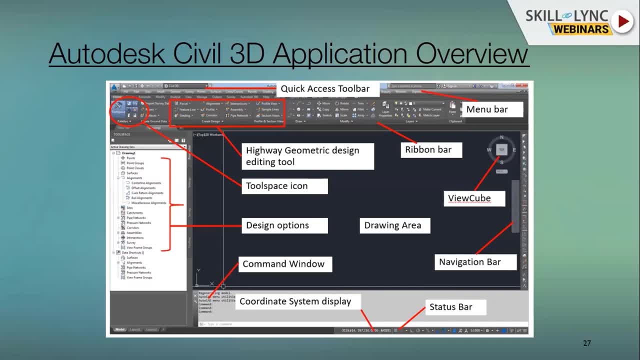 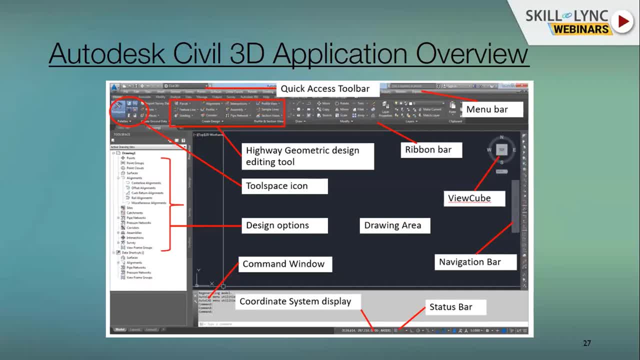 this presentation. so so once we open this application, you will be see all the parameters in the in the ribbon bar here, so this part of the bar is called ribbon by the top. Know the tab which says the file, edit, Insert. those are the. all the parameters will be called as menu bar. so the same parameters are there in the below with the details of this, all the tools which is now you can see in this, one so the other, what will be the quick tool access bar which you know, normal in excel, and what you can see, this: open file, the save as or open a new document. do undo those kind of parameters. 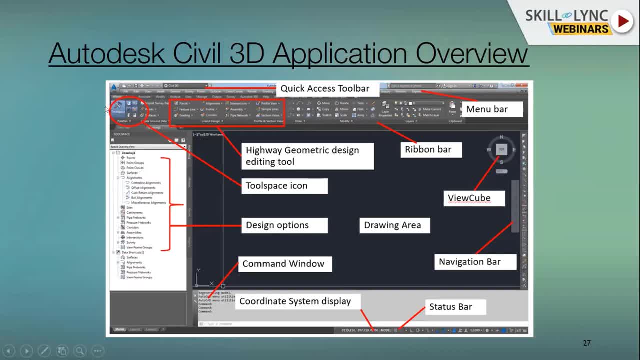 Will be there. so here is an important tab called tool space icon, which gives you This is the tool space icon. if you click this on and off, it will be showing this dialog box separately. so here is all the controls for this civil 3D. so I'll be explaining in the in the further slides how it will be. you know we use this one it is called. it has four sections here. one is prospector setting, survey and to the survey we don't use for normally because as a highway part we will take the survey directly from the. 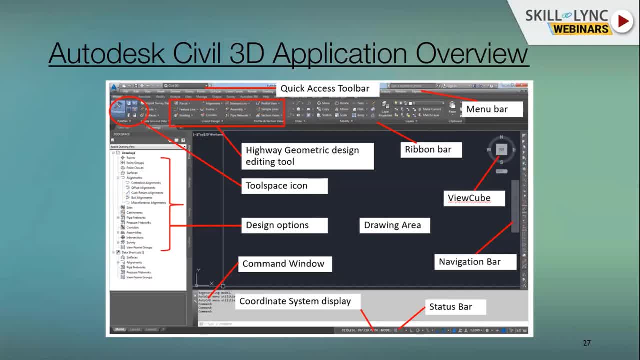 Surveyor or the survey consultant. we use that one. So the highway engineering will be using the prospector tab, setting step, and a tool bar tab. so these are the controls. we will do that. so, coming back, coming for the This Market section, you can see this will be the highway geometric design editing tools, so where we can create all the parameters, like you know, 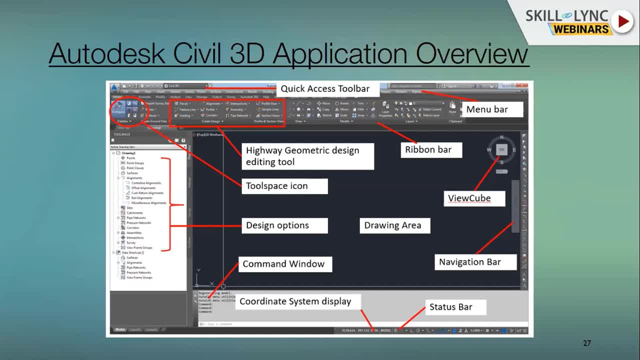 Alignment, design profile, design, corridor, intersections, assembly creations, You know no cross section developments, all those parameters will be controlled within this small area. it has a lot of features if you just you know, drop it down. so That's this one option. Quick, quick setting options we can see in this overview option. one background I would like to say here is civil 3D. isn't quite a bit of intelligent software where it understands the users, you know, requirement as such. 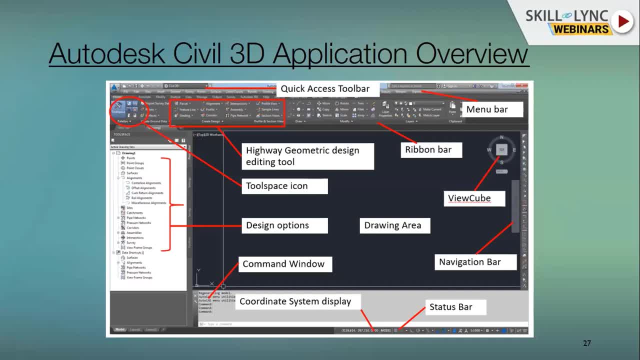 For example, I would like to say this: Because once we do it, as as in the in the table of content I said, the procedures like development of DTM, development of alignments and corridor and corridor sections, So finally the output, so all these features are the template, will be interconnected to each other. so if it says, once we design and we submit to the client and the client says no, no, I need to know, realign this, one argue the radius smaller or bigger. so once we do that,